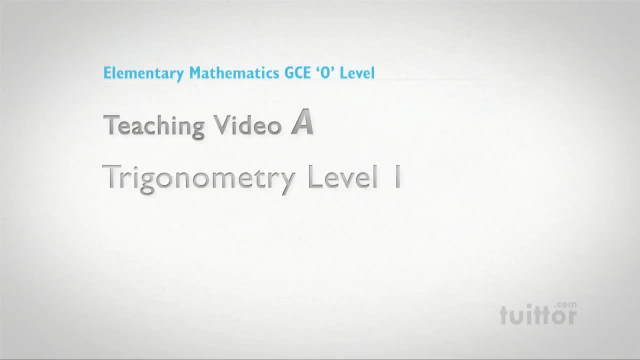 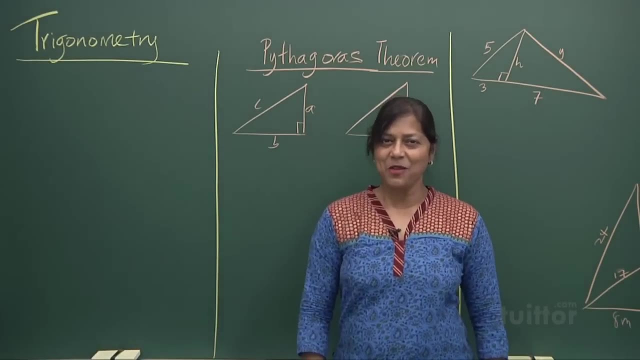 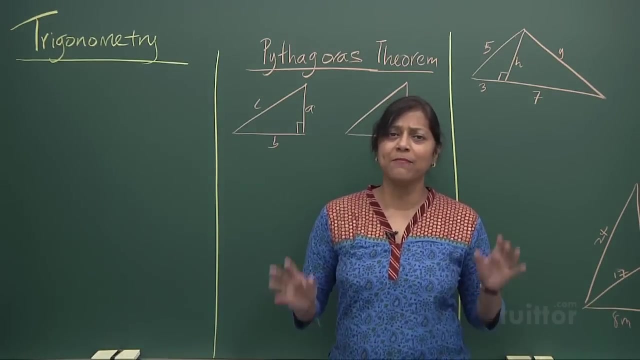 Well, how are you feeling Good? Are you game for meds- Meds with kumar will not be so stressful. let me tell you that, Alright, today we're learning something new on trigonometry, But have no fear, alright. 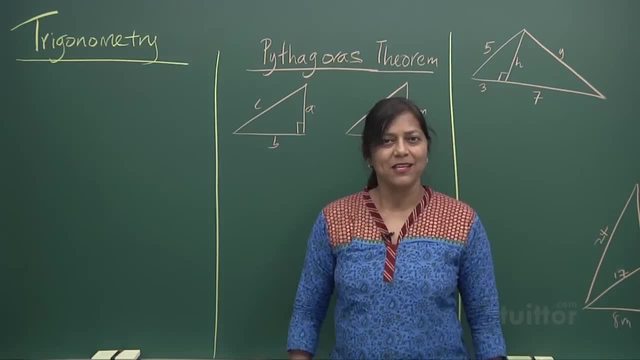 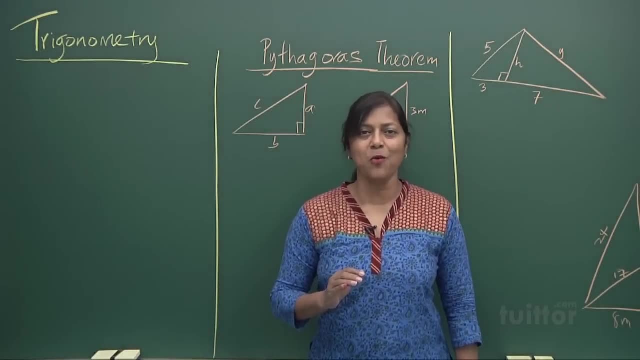 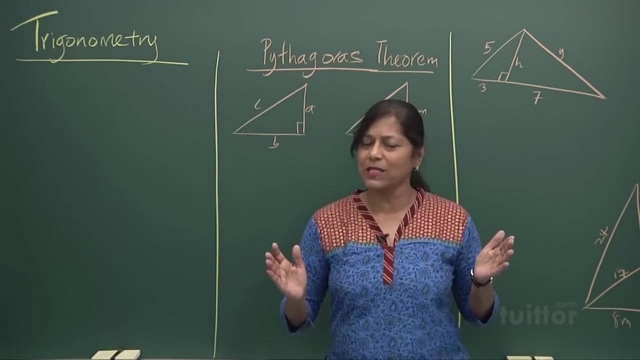 Alright, I'll take you through Trigo from scratch so that you will see and get to understand it in the easiest and best way, And you will get to know the importance of this chapter as we go along, because what we'll start is: what is Trigo, what's the use of it? 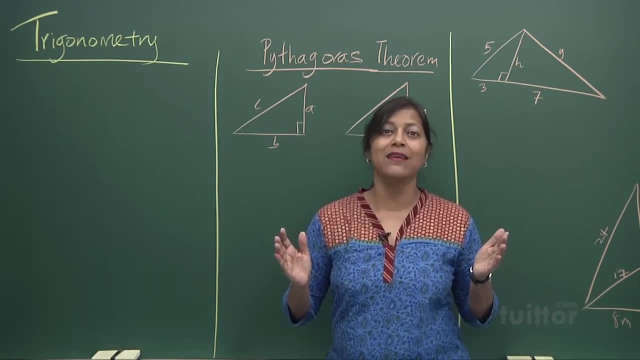 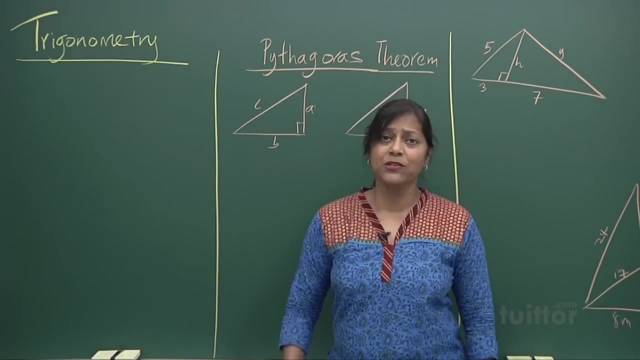 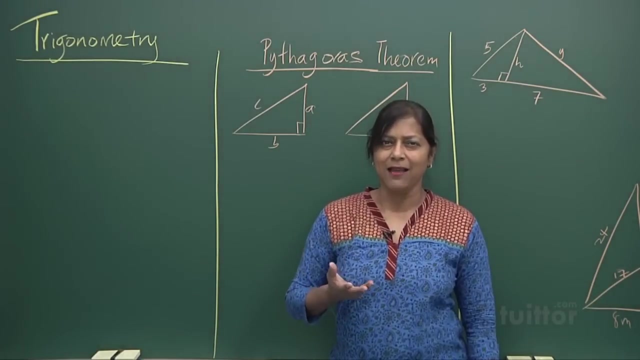 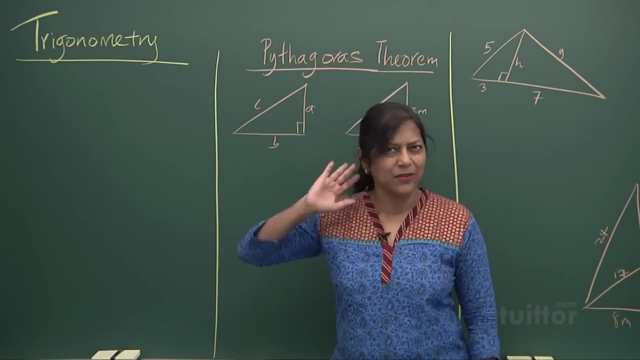 how do you use sine cosine tangent and how do you use these formulas in solving problems? And after which the next level will be the application of trigonometry in finding length, sides, angles, areas. And that's where you're going to get to sine rule and cosine rule. You've heard of it, haven't you? 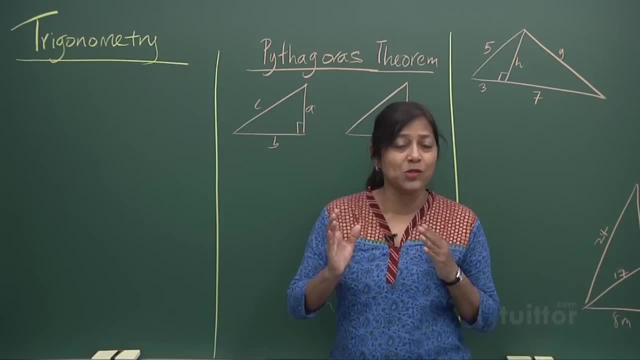 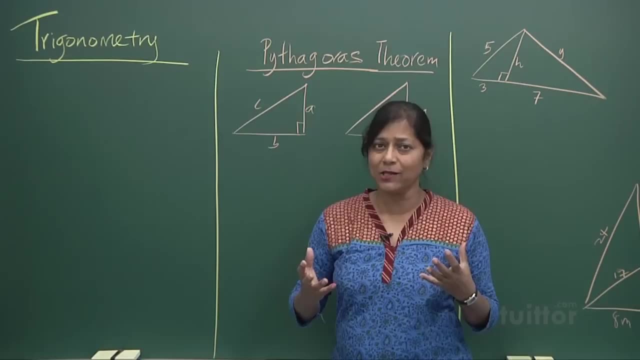 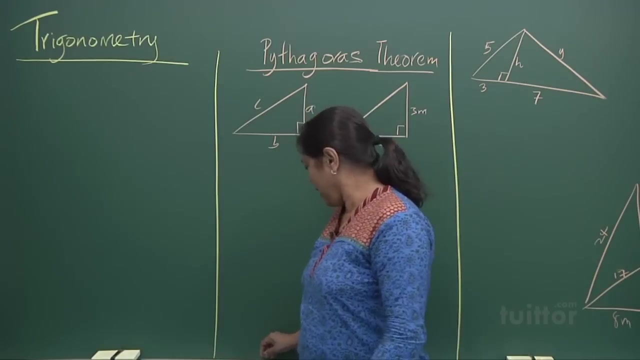 But don't panic. Once you get to know about it, as you develop from stage 1 to 2 to 3, and you get to bearings, alright, With all this fundamental knowledge you will be up there, Alright. but just before we get to Trigo, I'd like to revise with you a general revision on Pythagoras' Theorem. 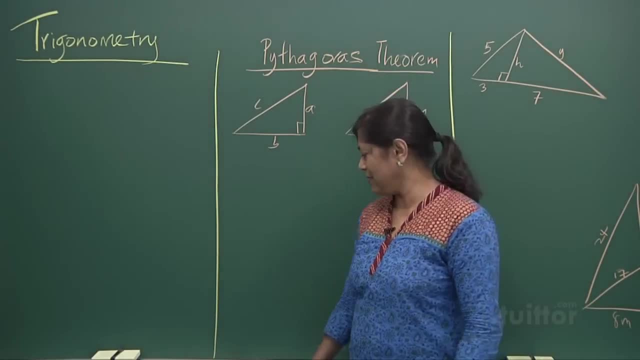 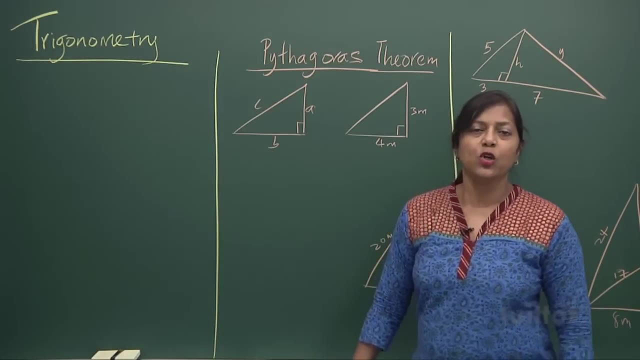 What is Pythagoras' Theorem? And if you look at this, you look at a triangle, here triangle, and you have A, B, C. You call the longest side the hypotenuse. Please don't call it hippopotamus, alright. 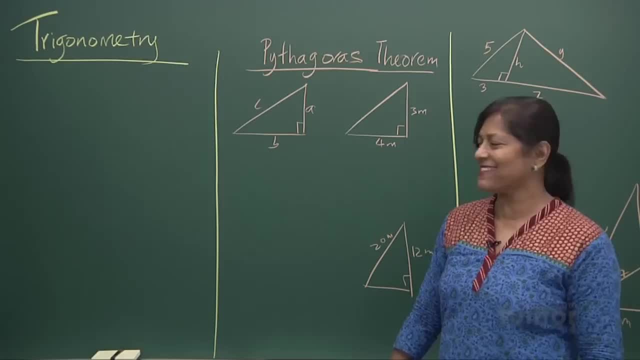 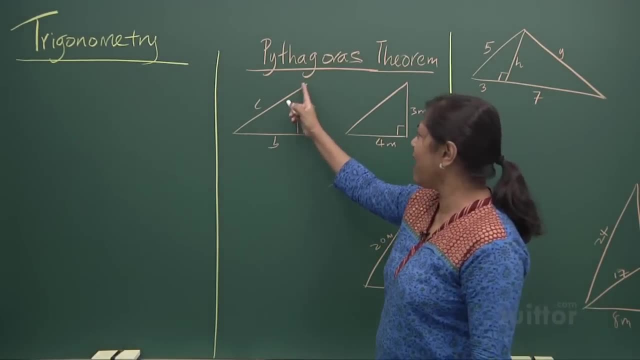 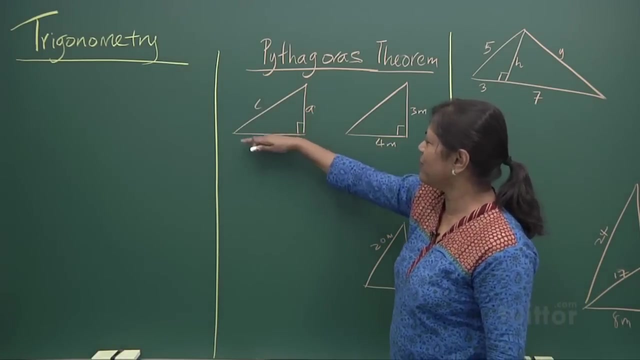 You call it again hypotenuse. Yes, Now, this is the hypotenuse And the hypotenuse. how do you recognise it? It's the side that faces the 90 degrees, That's facing the 90 degrees. These are just adjacent sides to 90 degrees. alright, 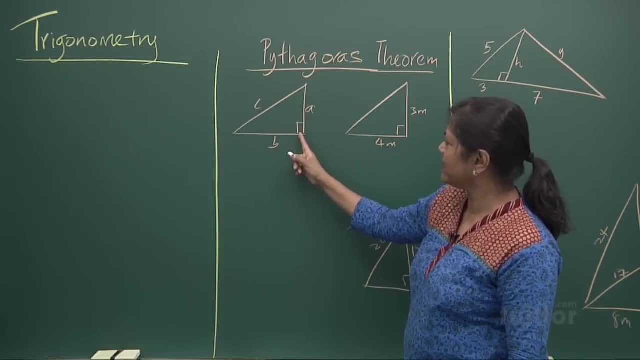 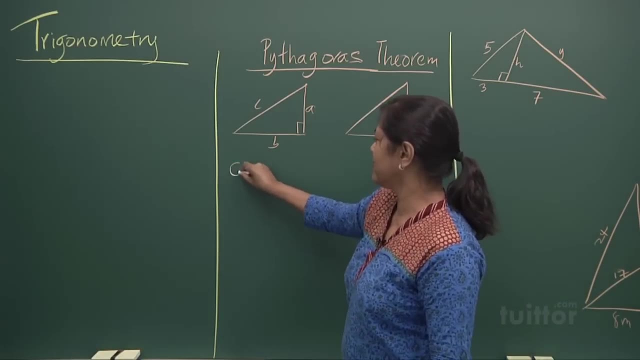 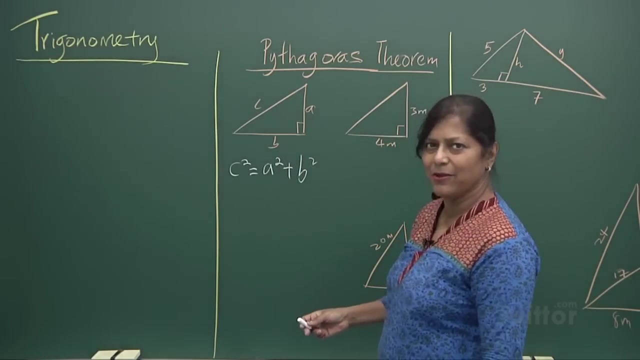 Now, the hypotenuse facing the 90 degrees is the longest side of the triangle And it's made of C squared. It's none other than A squared plus B squared. This is Pythagoras' Theorem, And amazing. you just draw it out in your paper. 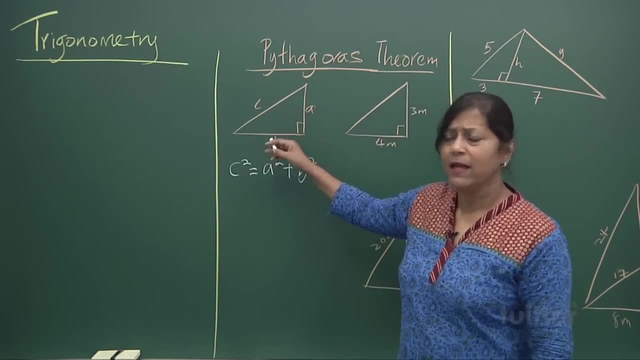 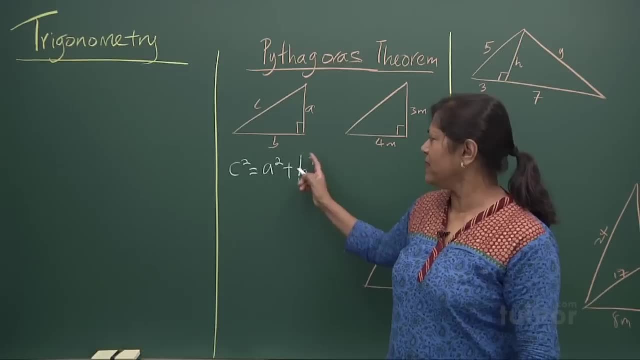 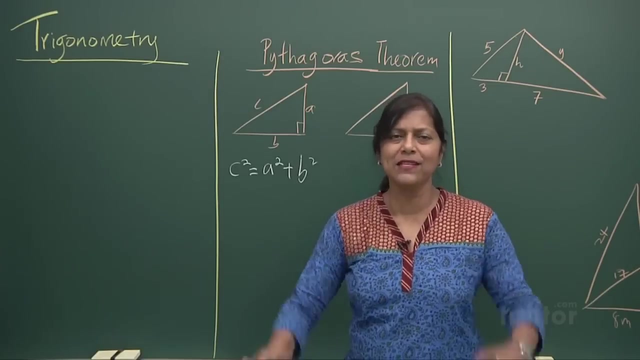 Just draw any right angle, Measure the side here, measure this side, Square them like what you did here And see if it is the sum of this, if it's the square of this length. Alright, You will discover that, And no matter whatever size your right angle is. 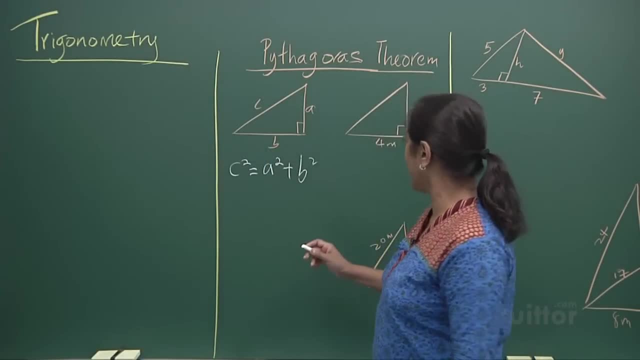 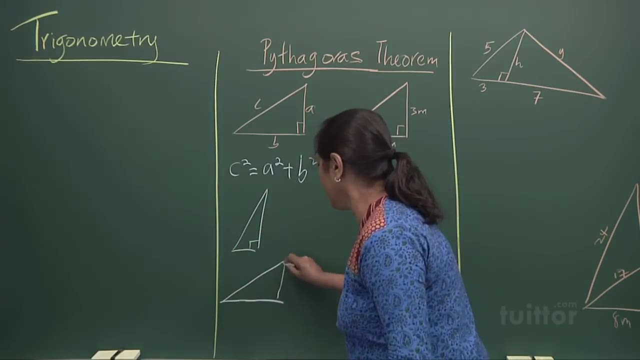 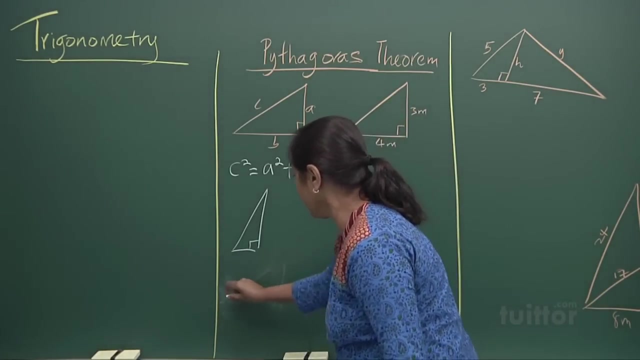 no matter how small, big, whatever, you can draw a triangle that is very thin. this way, You can draw a triangle that's very big this way. Alright, Let me draw another one, A triangle that has got huge length here and very short length here. 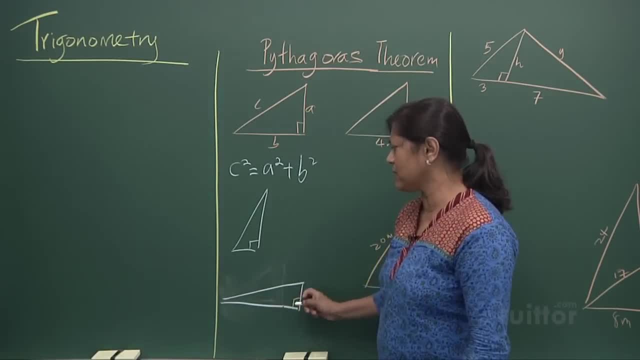 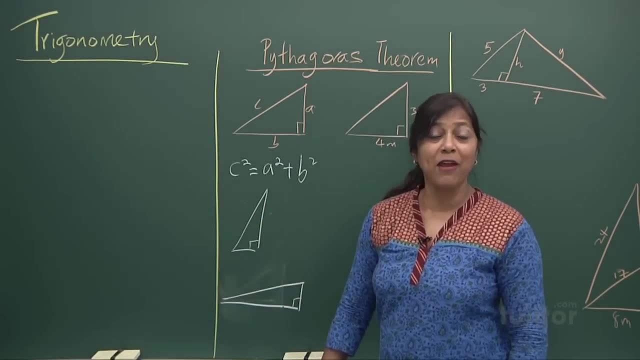 Alright, Whatever it is, the square of these two distances will be equal to the hypotenuse. Alright, The hypotenuse is here And I think they rightfully called it right hypotenuse Because it looks like the hypopotamus of the triangle. 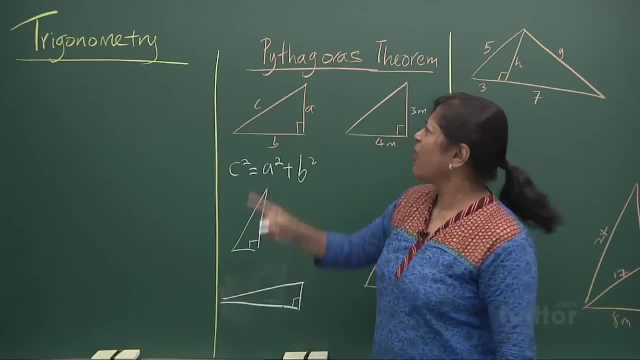 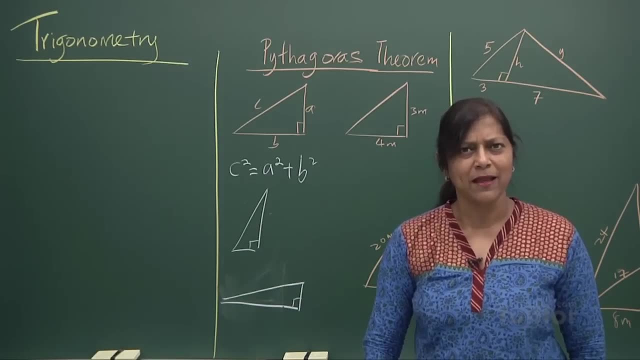 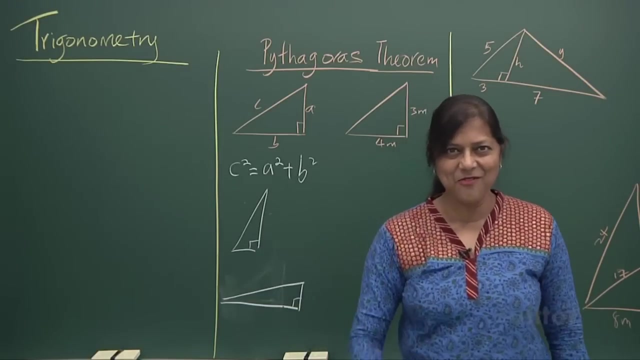 Alright, Hypotenuse, hypopotamus, God knows, maybe Pythagoras, this gentleman, find out more about him. He could have linked it that way. How did he get this name? Ah, perhaps you can do a finding on that and share it with me, if you can. 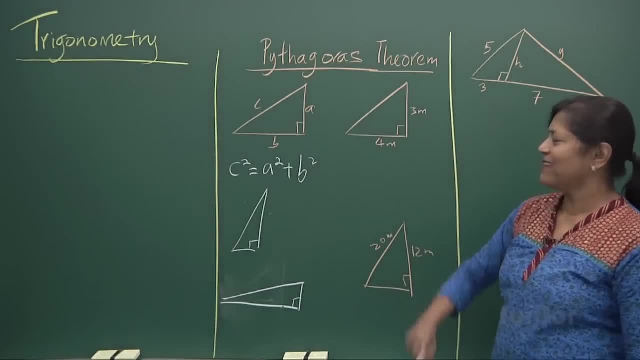 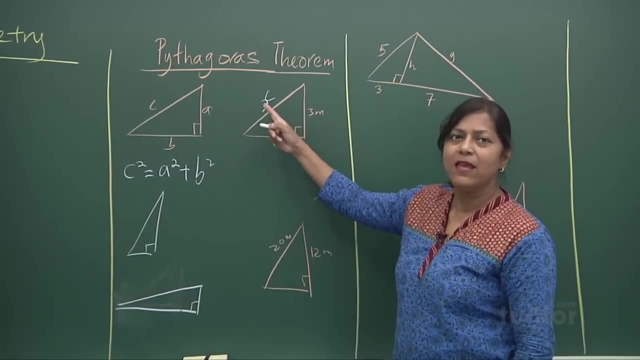 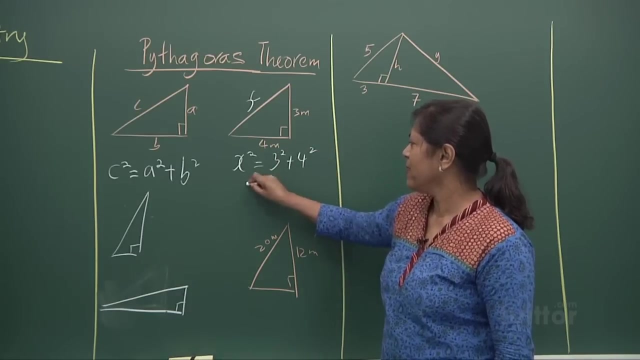 Kumar. Alright, let's look at this. You need to find out what is this length, if you remember? Ah, 3 squared plus 4 squared equal to x squared, So x squared is going to be 3 squared plus 4 squared. 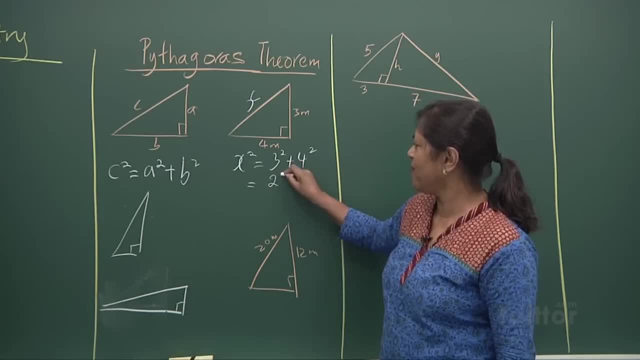 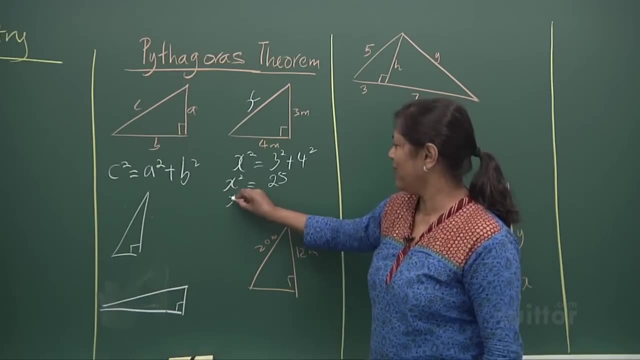 9 plus 16,, you get a 25.. And hence your x will be the square root of 25.. That is a 5.. Okay, Now, if you look at this triangle, you have 20 meters. Here is 12 meters. 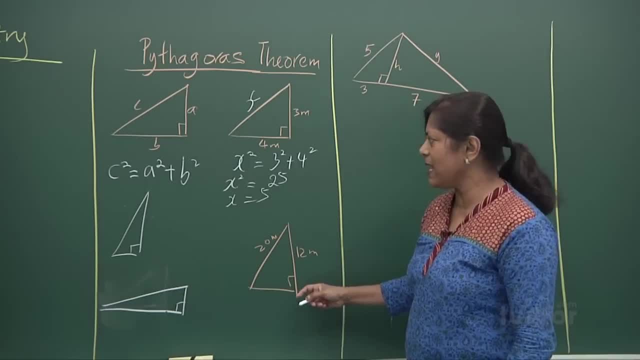 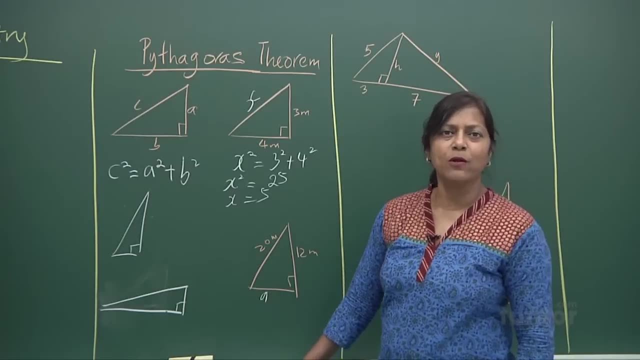 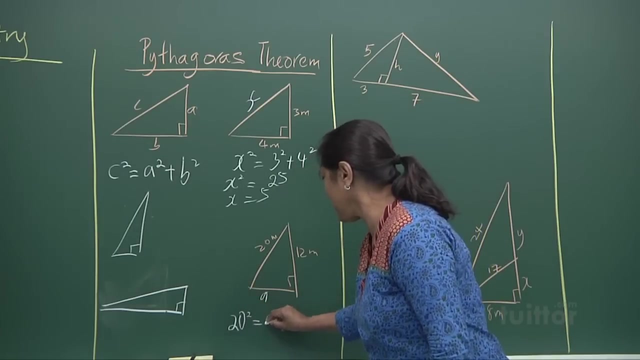 What's the length here? Give it a name, Call it maybe A. These are sides You've got to recognize where your hypotenuse is. Ooh, that's there. So 20 squared is none other than A squared plus 12 squared. 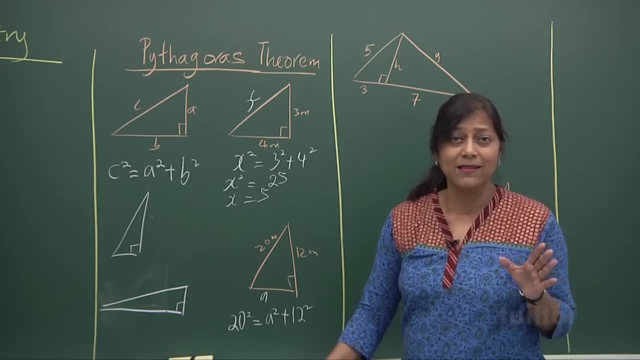 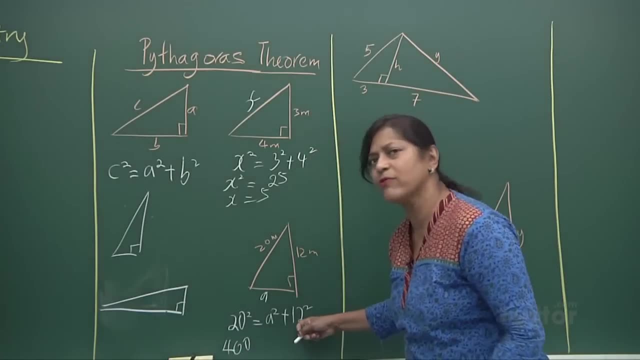 And you've got 20 squared, 20 times 20.. Pretty easy, 2 times 2, 4.. And you get two zeros there from here, So it's 400.. And if you look at 12 squared, 144.. 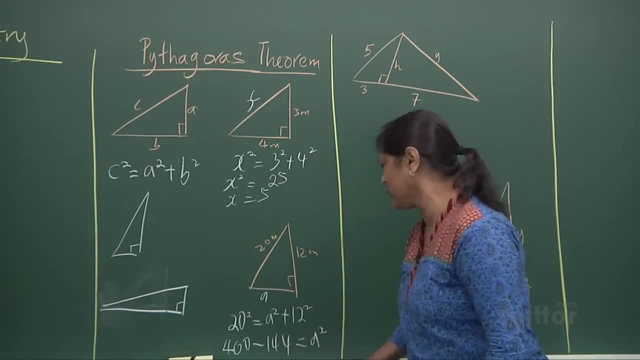 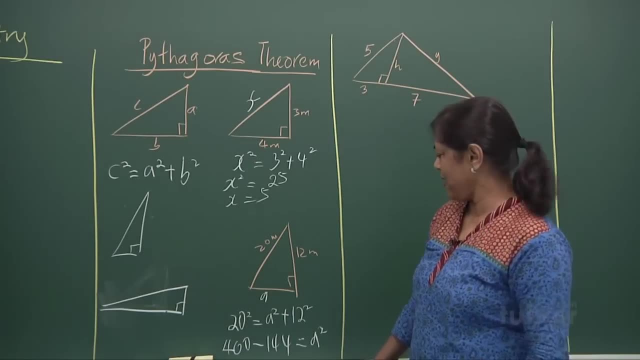 You minus your 144. What do you get? Your A squared to be Alright. Look at it: 400 minus 100. You have 300. And then from there, you've got a minus of 44. You get 256.. 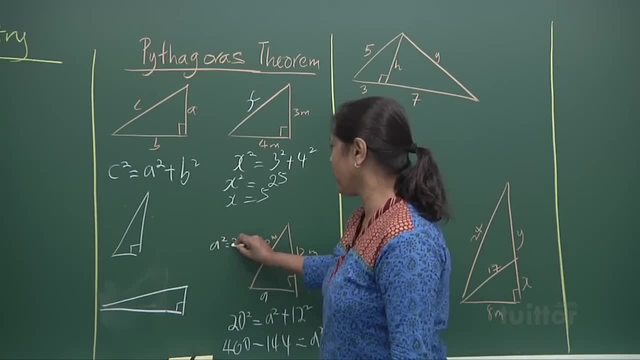 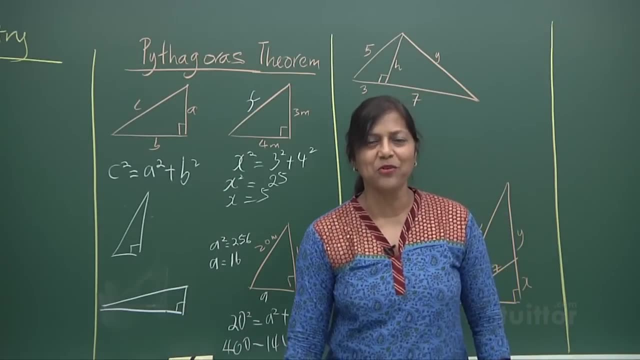 So your A squared will be equal to 2.. 5, 6. And the square root of it will be 16.. I know, when you find square root you've got a plus 16 and a minus 16.. Can the length be a minus 16?? 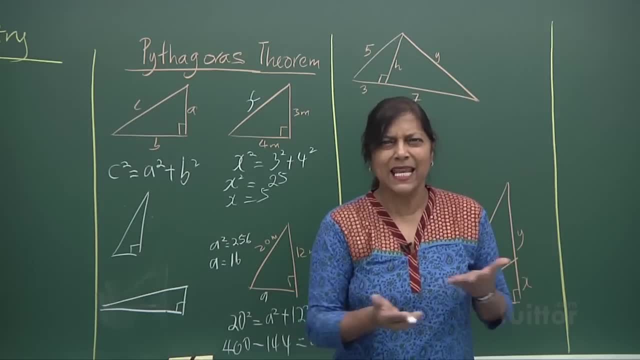 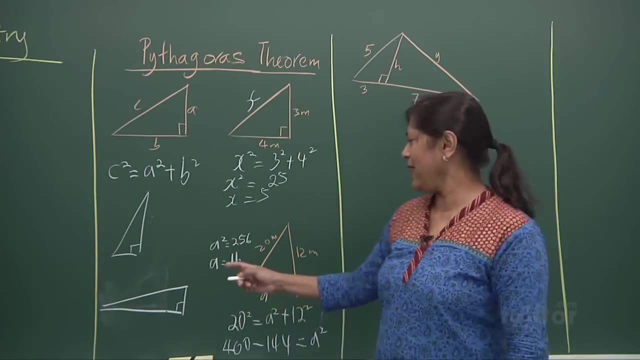 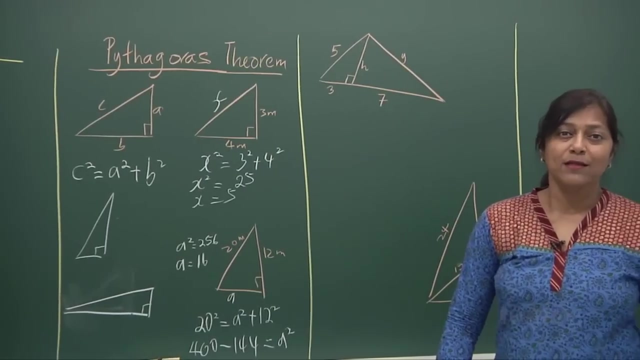 Where does that go? Minus 16.. Can the length ever exist? Where is the minus 16?? That's when you totally say reject, So A is 16.. Alright, Let's look at another few more examples before we move on to trigonometry. 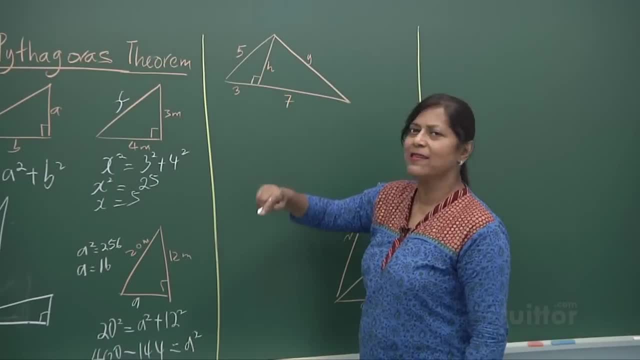 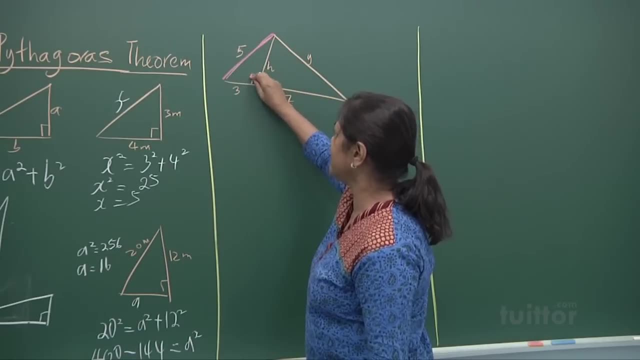 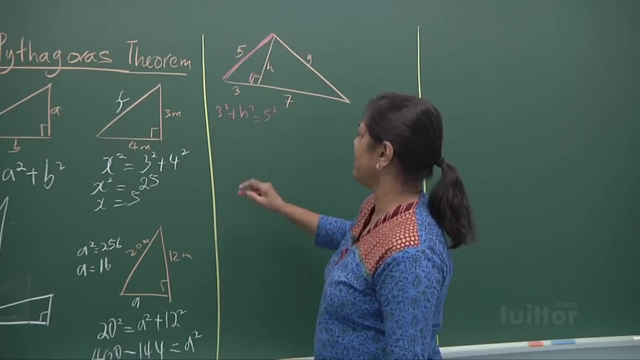 Alright, Now you look at 3,, 5, and this is H. What is H going to be? Well, this is going to be the hypotenuse facing the 90 degree. Alright, 3 squared plus H squared is 5 squared. 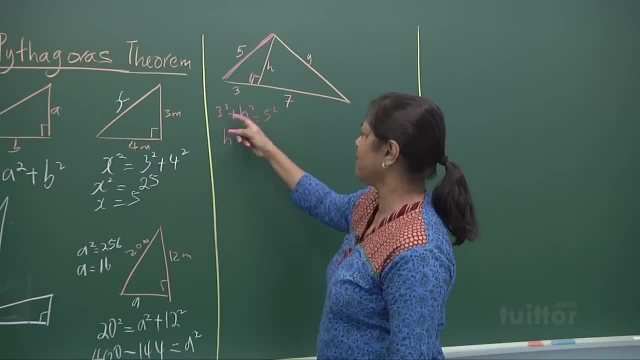 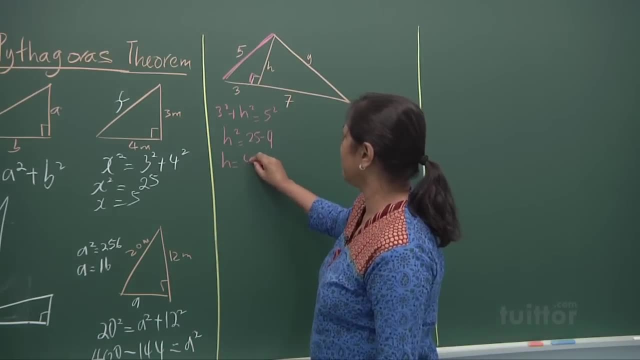 And that means your H squared will be 25, take away 9. And that's equal to 16.. So your H is going to be 4.. And if this length is 4,, alright, what is Y going to be? 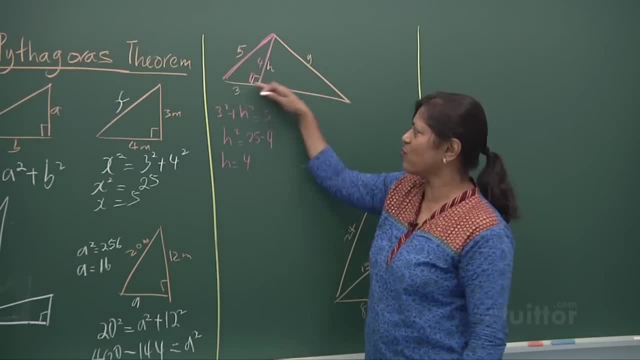 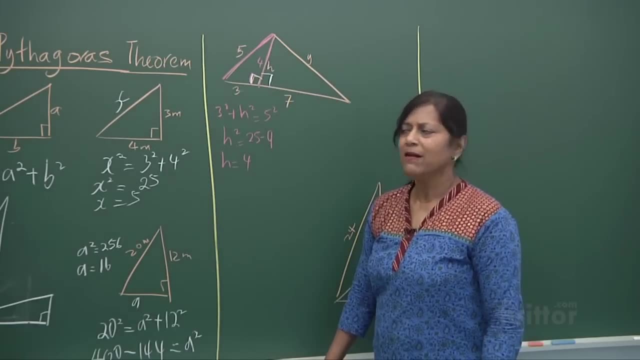 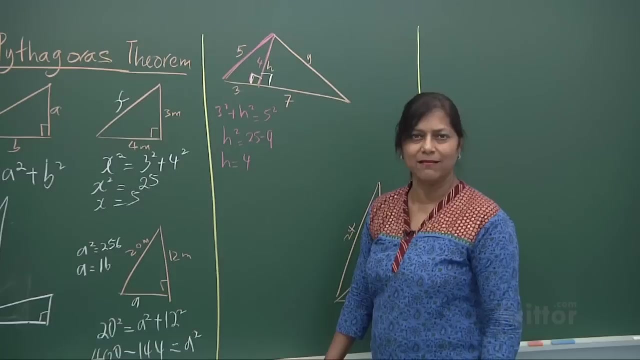 Now, these are adjacent angles on a straight line. If you have 90 degrees here, this will also be 90.. Now remember the very condition for Pythagoras' theorem: It must be a right angle triangle, Not in any other triangles. 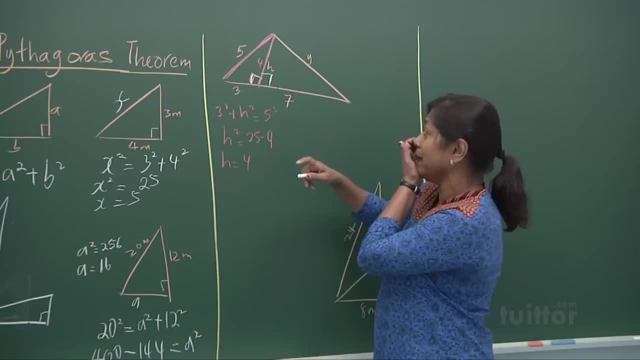 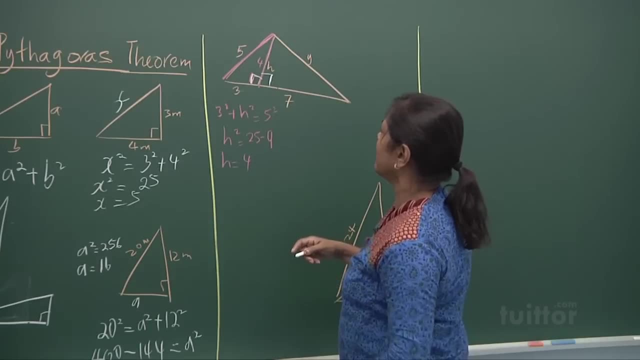 Alright. So that's why we created a right angle triangle here. And you have H, you have 7, and you want to find out what is Y. Alright Now, and it's also if you can do that, you can find out what is Y. 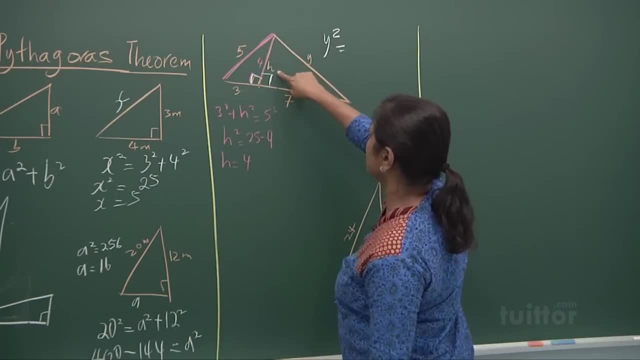 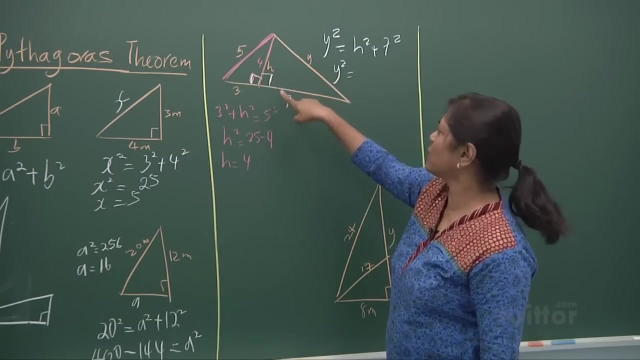 Your Y squared is going to be H squared plus 7 squared, And so your Y squared is going to be: look at that- H squared plus Y squared. Y squared, sorry, is H squared plus 7 squared. That's the hypotenuse facing the 90 degree. 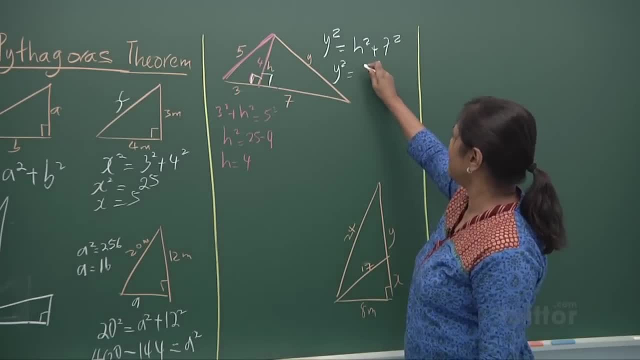 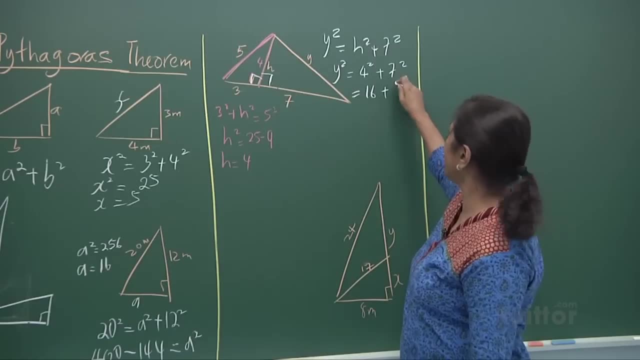 Right. So look at it: Your H is a 4 squared 7 squared a 16 plus 49.. When you add that up, what do you get your Y to be? Please help me there. 50, 56.. 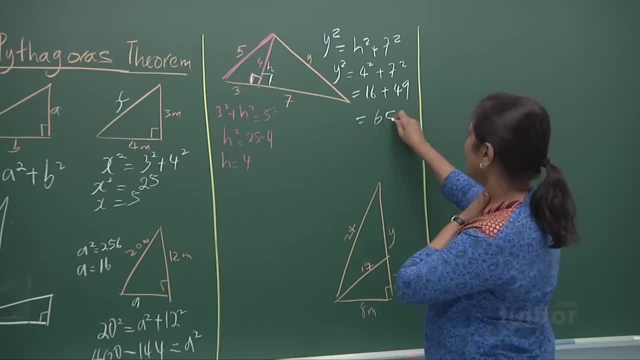 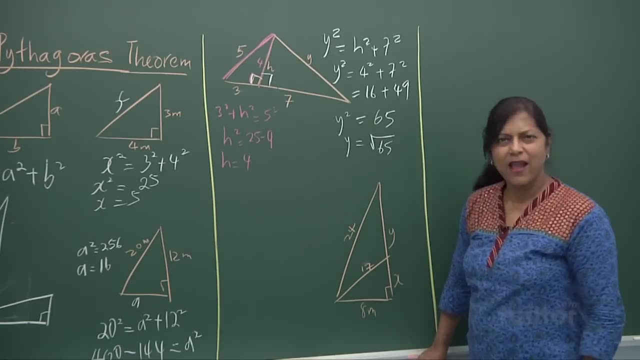 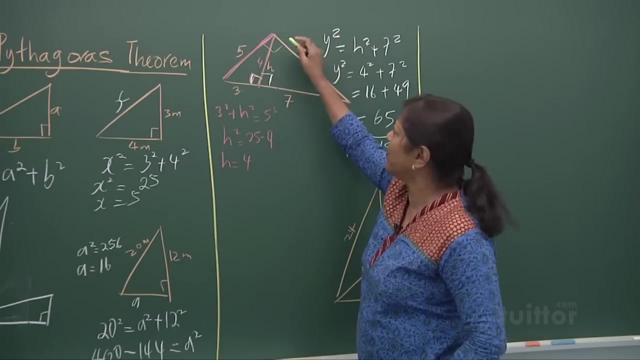 65.. Right, That's Y squared And Y will be the square root of 65.. Have I made a careless mistake? No, Right, Okay, So you've got Y the square root of it. Now we wonder. I want to ask you: can this angle ever be 90 degrees? if you want to find out, 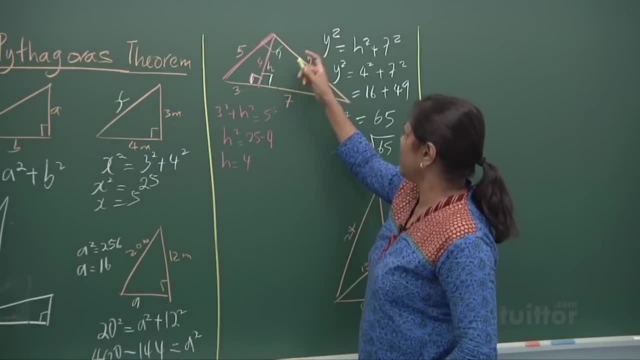 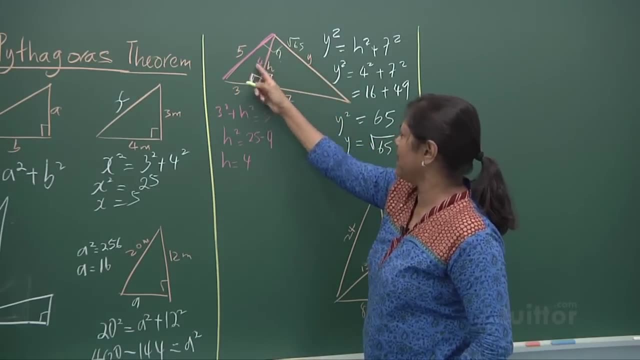 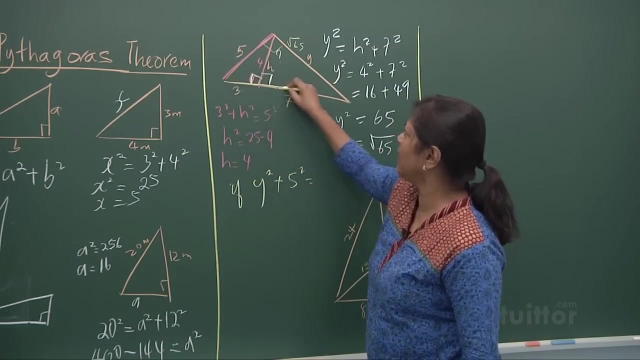 Is it so? If it's so, then if your Y is a square root- 65,. this should match. If this square, Y squared plus 5 squared, if your Y squared plus 5 squared is equal to this whole length, 3 plus 7 is 10, 10 squared. 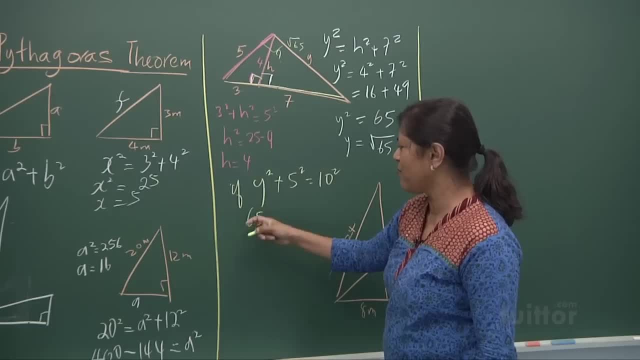 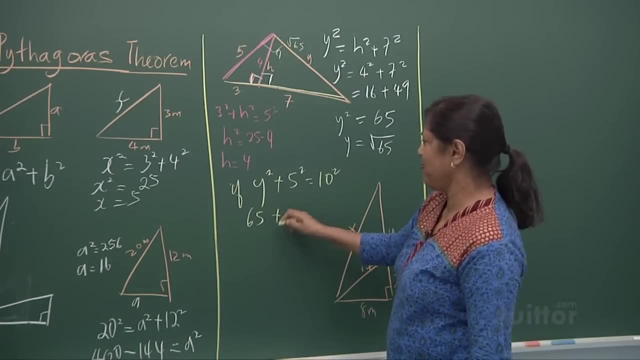 If let's find out, that's 65 square root. when you square root, square root 65, you square it, it becomes 65. And this is 25.. You want to find out And this: you get 80,, you get a 90,. 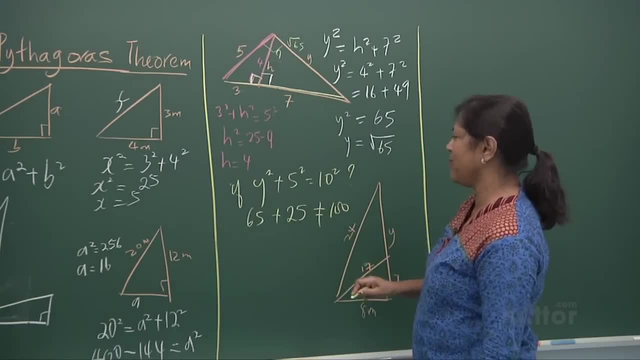 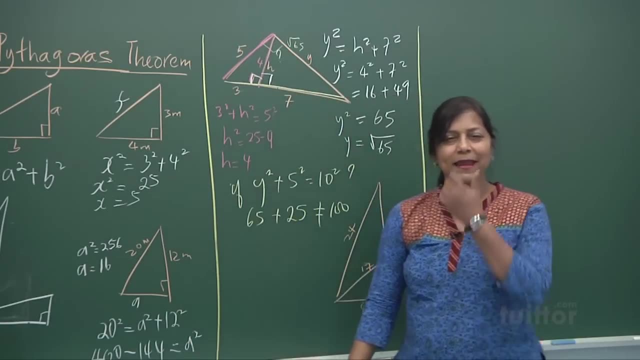 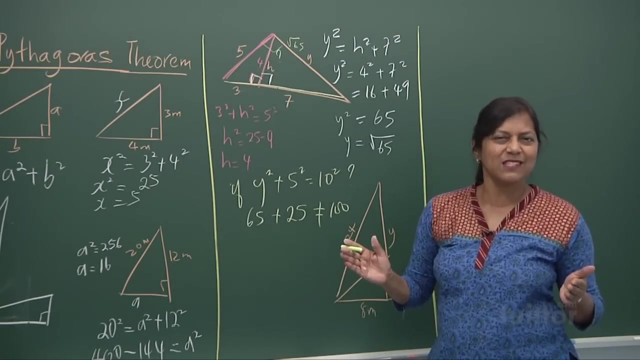 and a 90 is not equal to 100. Hence this angle here is not 90 degrees. All right, So you want to test it. if it's 90 degrees, it must be following Mr Pythagoras his theorem. 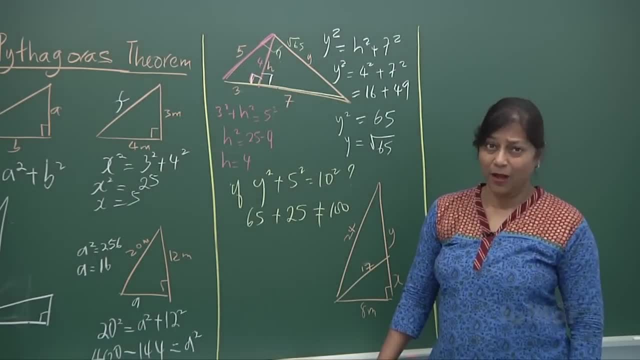 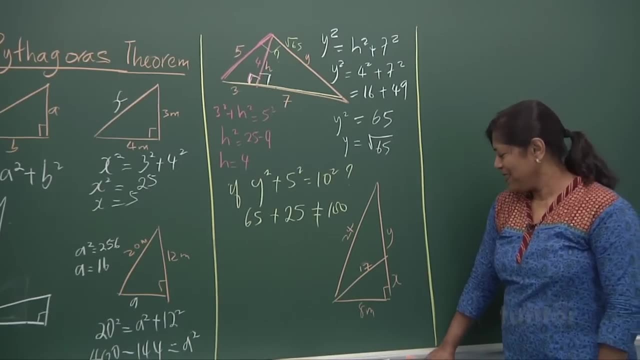 All right, Pythagoras' theorem: Mm Got it Right. We can move on a little bit, and then I'm going to get to trigonometry. Now you look at this again, You've got an 8.. 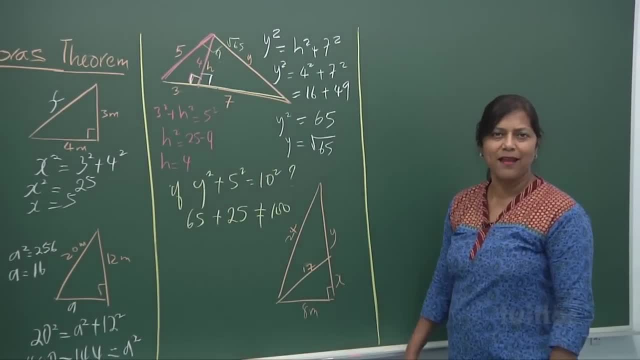 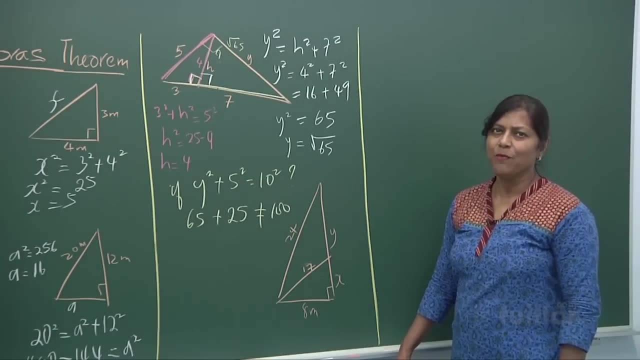 You've got a 17.. You want to find out your X? You want to find out your Y? Are you comfortable with this? I always tell my students, those who come to me, I said: hey, don't be a nerd, you know. 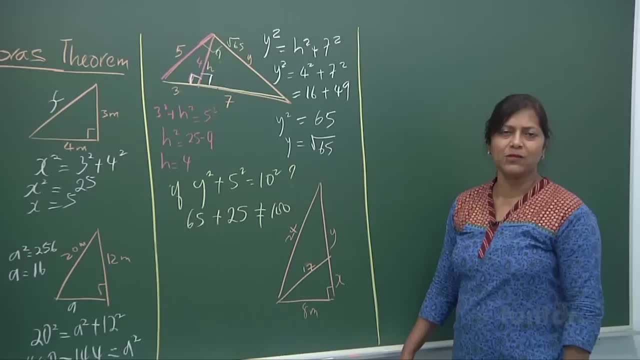 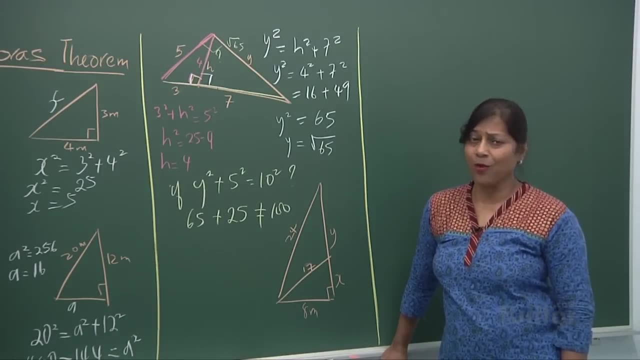 Don't rely on the calculator too much. Know your tables, Know your squares, From 1 squared to 25 squared. 1 squared to 25 squared Like what is 13 squared 169.. What's 14 squared? 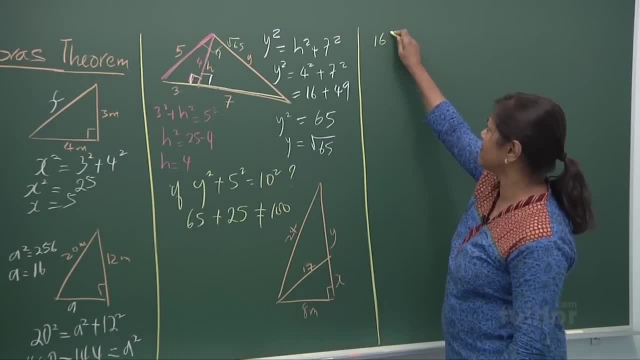 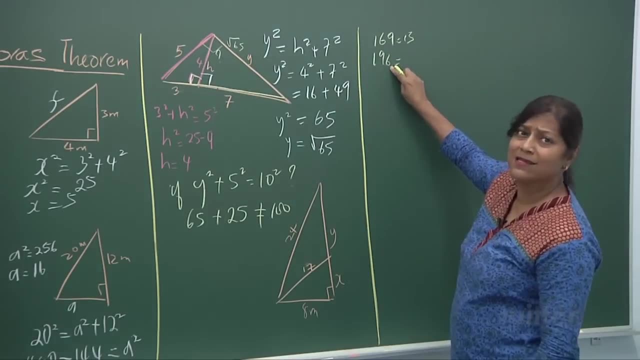 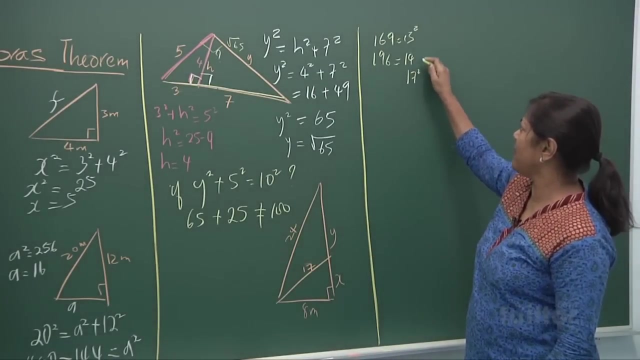 Look at the amazing figure of numbers 13 squared. That's that 14 squared, Reverse the numbers, 69 becomes 96.. Hey, that's 14 squared. And you've got to see patterns Like if you look at 17 squared. 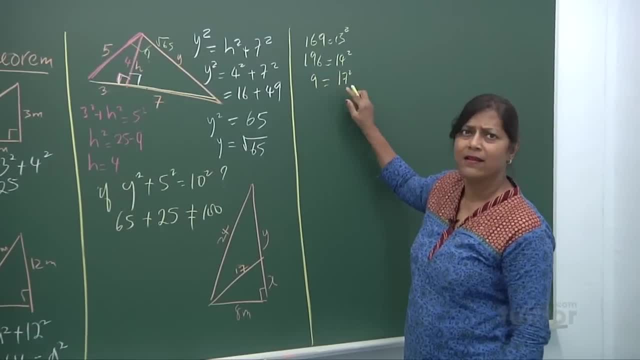 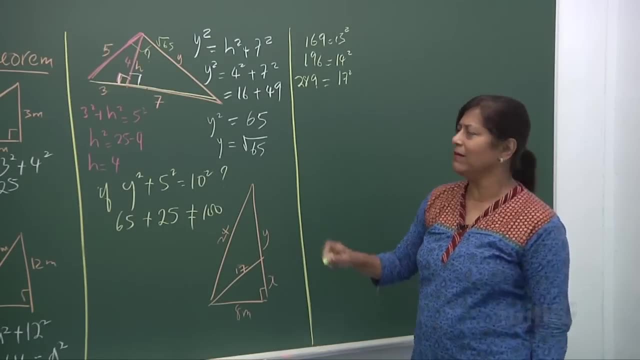 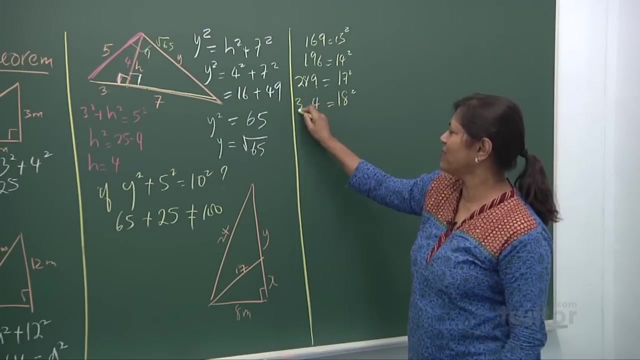 Now you look at 7.. It ends with a 9.. 17 squared, It is 289.. It's not very difficult. If you look at 18 squared, It ends 8 times 8? 64.. And these two numbers you've just got to remember. 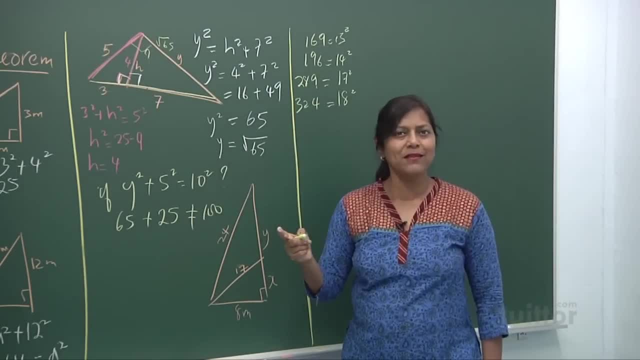 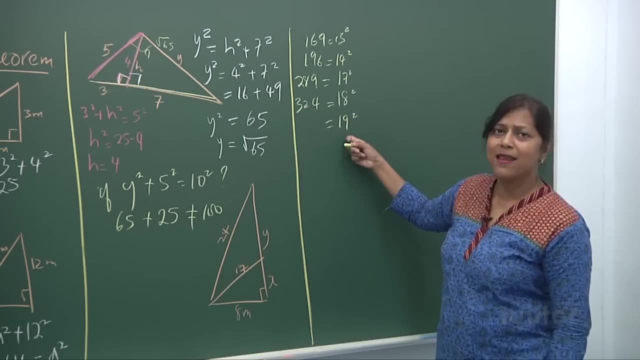 It's more than 200.. Less than 400.. Well, it's 300.. And this center number is what you've got to remember, And 19 squared 9 times 9. It's 81.. It can't be 4 for the hundreds. 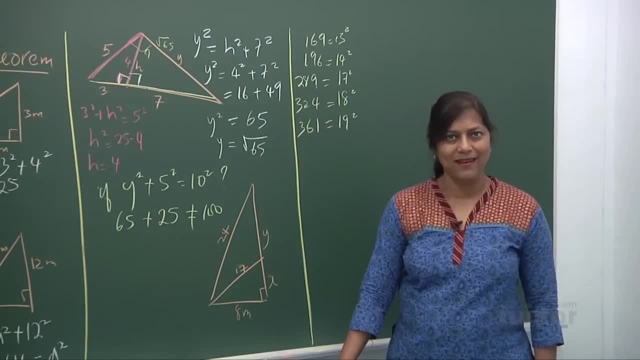 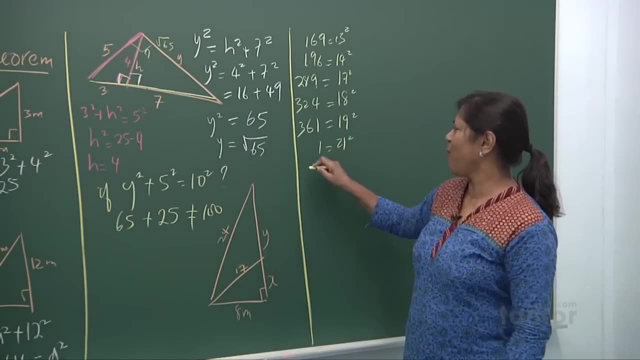 It's 3.. And this is 361.. 20 squared, I'm sure you know, And 21.. Similarly, if you look at 21 squared, You know it's 41.. It's more than It's slightly more than 400.. 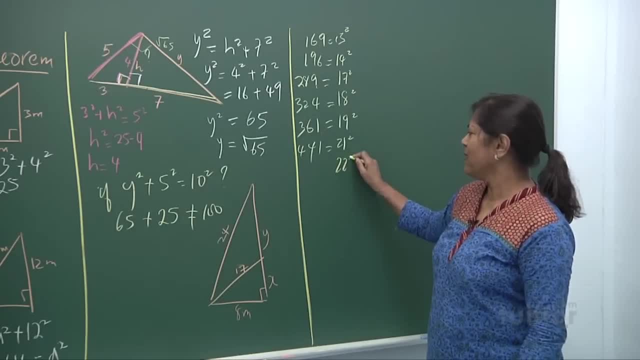 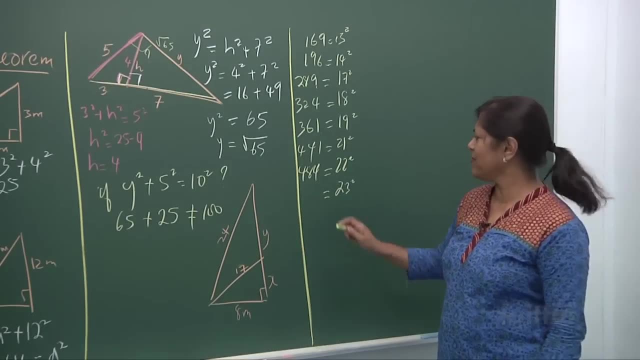 You get 441.. All right, Move on with grace. You can see, at 22 squared It's 484.. 23 squared, If you can help me there, Is it 576?? I think so. Wait, No, no, no. 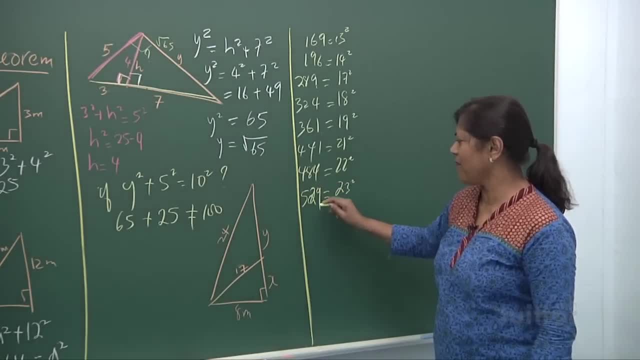 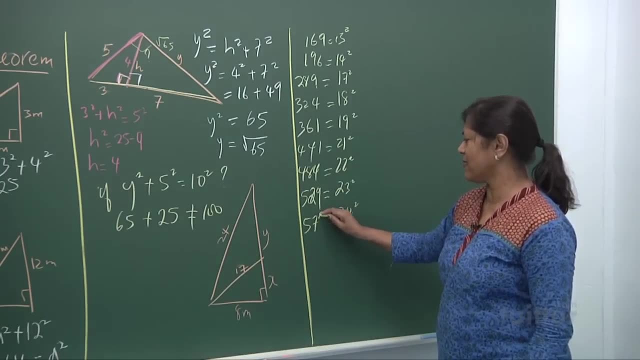 3 times 3 is a 9.. I think it's 529.. All right, And if you look at 24 squared It's a 576.. And at 25 squared It ends. You look at 24 squared again. 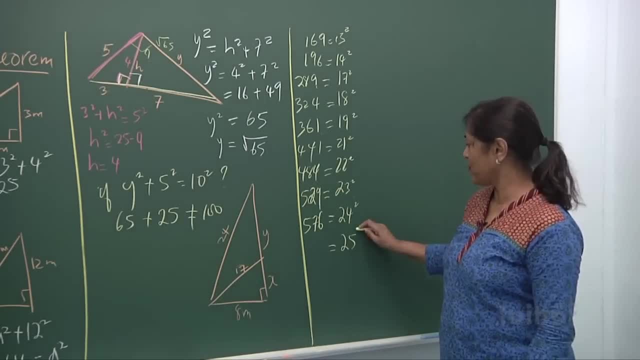 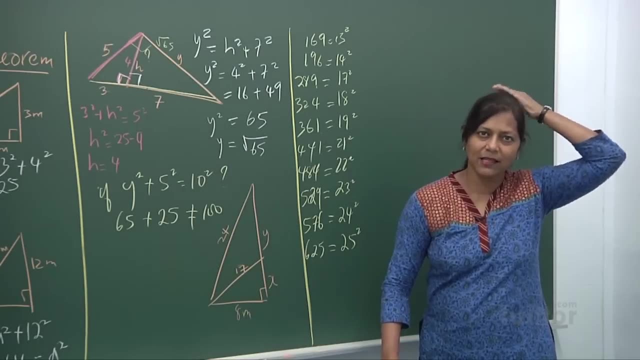 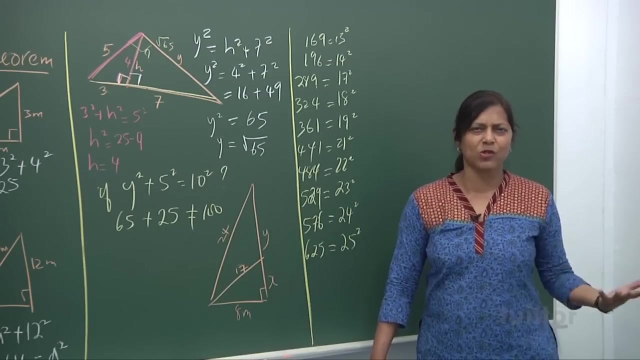 4 times 4 is a 16.. 25 squared, It's 625.. It's good to have all these in your head And just like the cubes- from 1 cube to 12 cube- It will be really good, Especially when you have to find so much of square roots and all these. 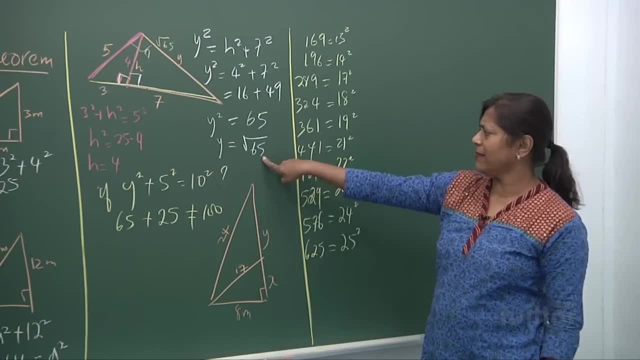 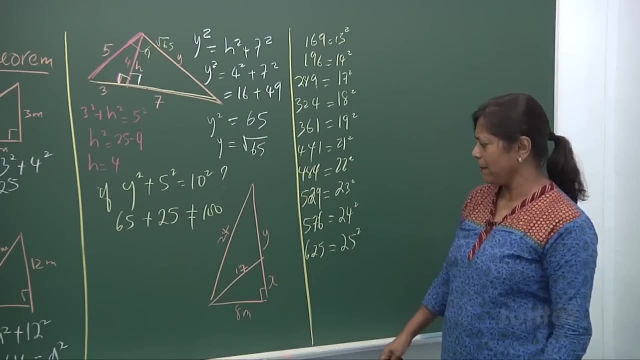 You have an approximate picture, All right. This length is about 8 point something. Square root of 65 is about 8 point something. Now you look at this. You want to find out what is x. All right, What do we do? 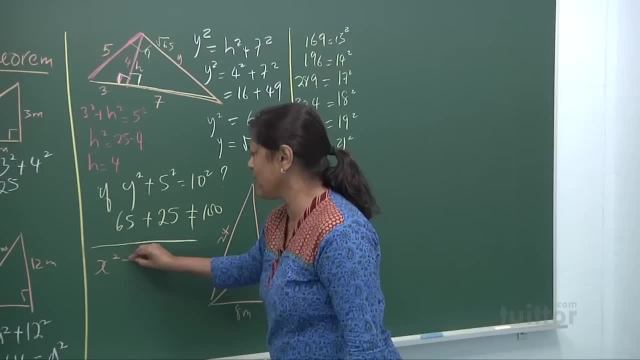 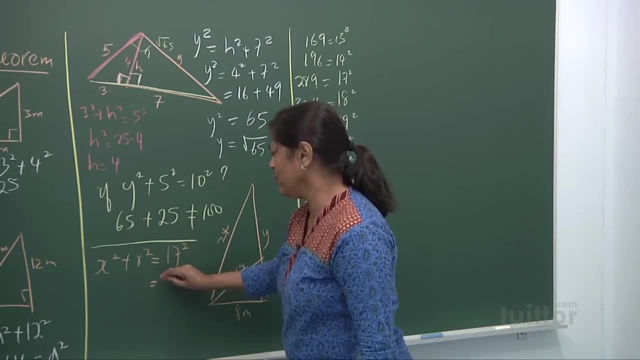 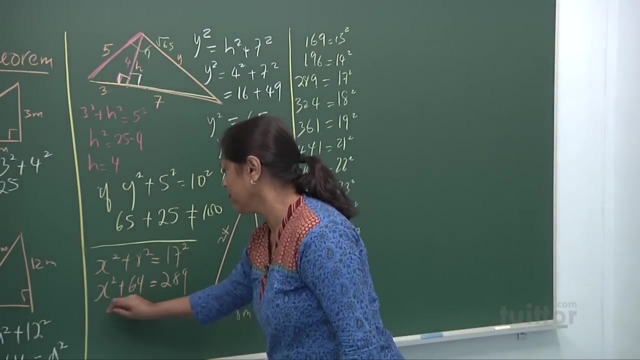 We said: x squared plus 8 squared Is equal to 17 squared. And you know what is 17? 289.. And this is 64. So you got to bring that over. Your x squared will be 289.. Minus your 64.. 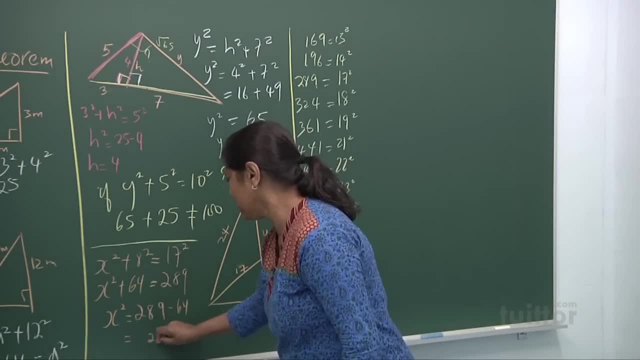 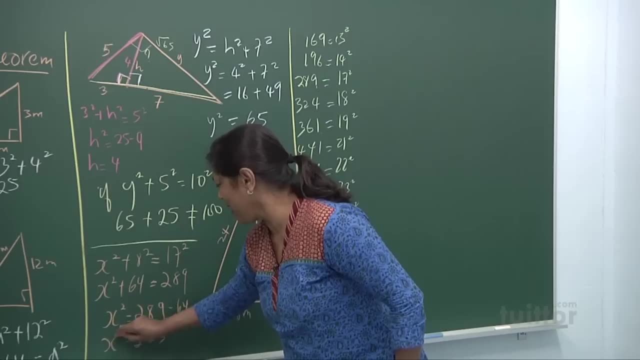 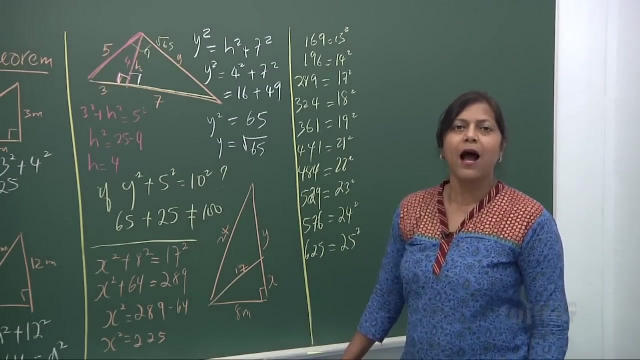 And that will give you a 5. A 2. A, 225.. All right, That's an interesting figure. X squared is 225.. And what is 225?? The square root of it, 15.. I remembered. I must share this joke with you. 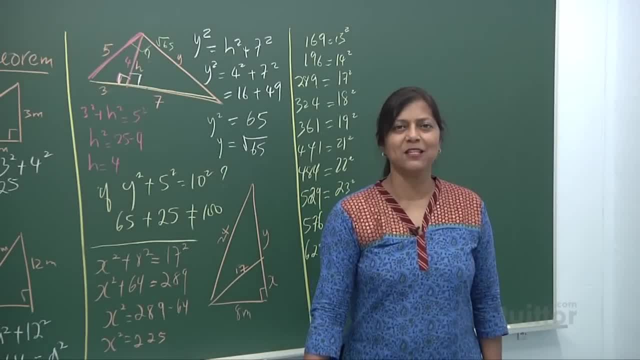 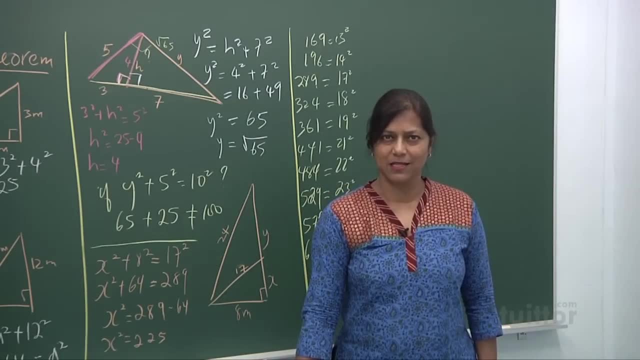 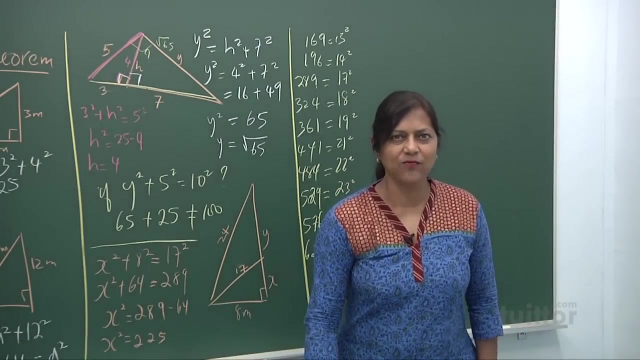 Don't laugh too much And keep it silently to yourself. I was teaching at one of the schools some years ago- A good 20 years ago- And I was quite scared of this huge, strong guy who sat in front of me. I asked him: what is 5 cube? 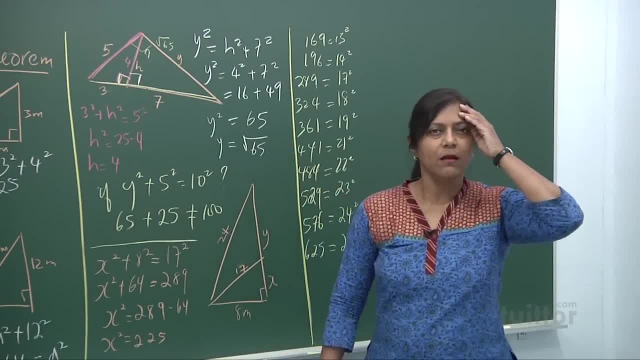 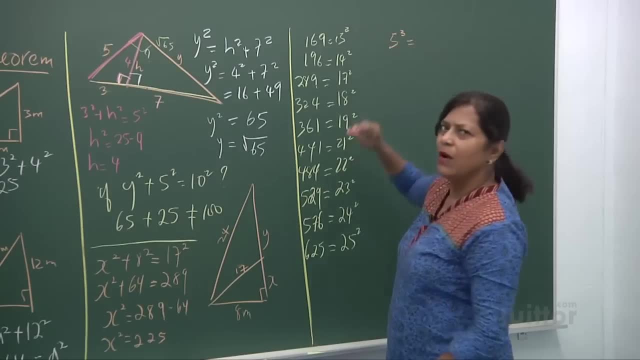 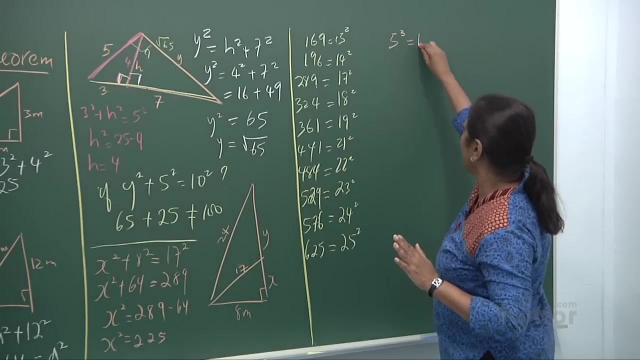 He looked at me and he shouted: 125.. I said what 125?? He wanted to fight with me. All I asked him was 5 cube, 125?. I said what again 125?. I heard it that way, But actually he was saying 125. 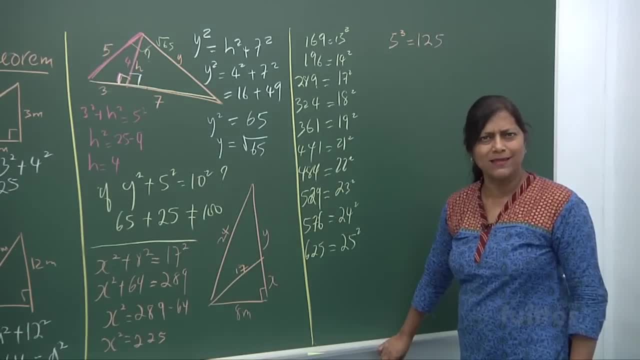 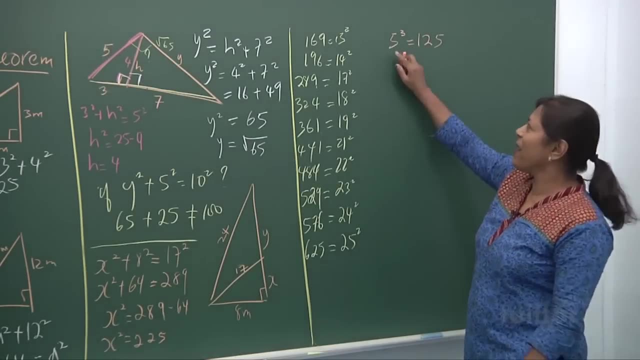 I got that. I was a little worried for once. All right, Not now anymore. I've become a much more mature teacher. I can take it on. All right, 5 cube 125.. 125.. Remember the fight? 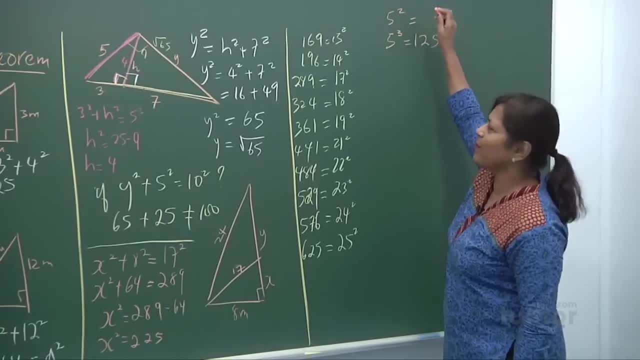 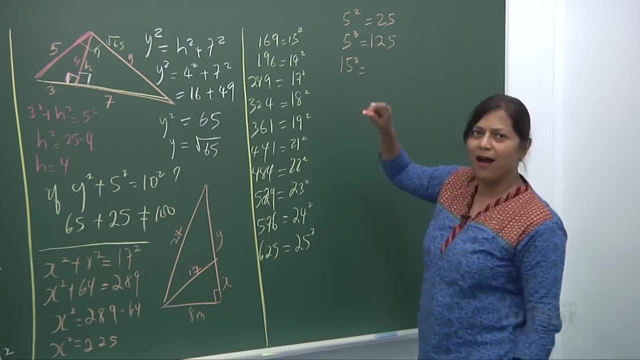 To fight: 5 squared. So I got this as a little hamper To fight To fight And I said 15 squared. Ah, 1 to fight, 2 to fight. Oh, This is dual fight: 2 to fight. 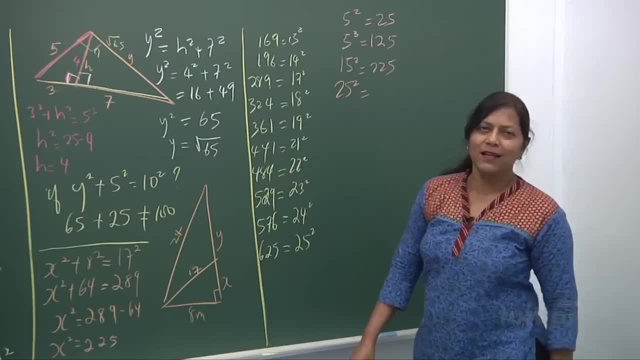 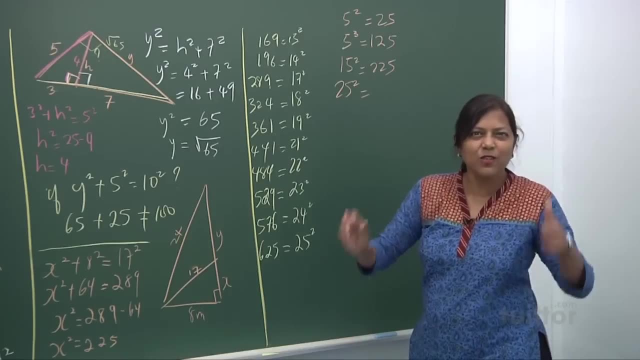 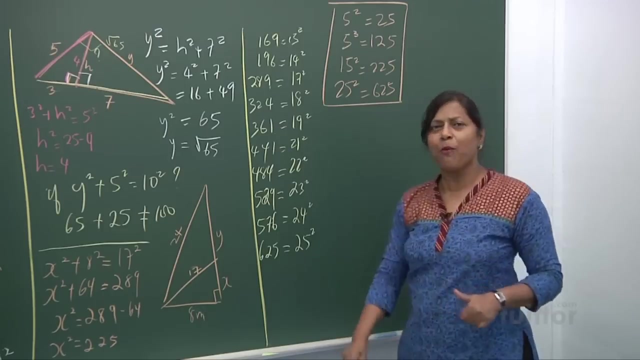 And I said: 25 squared. Oh, It's a gang fight. What do you guess it to be? All right, 6 to fight, 6 to fight. That's how you connect numbers with your own version, And I thank this lovely boy actually for teaching me how to be a better teacher. 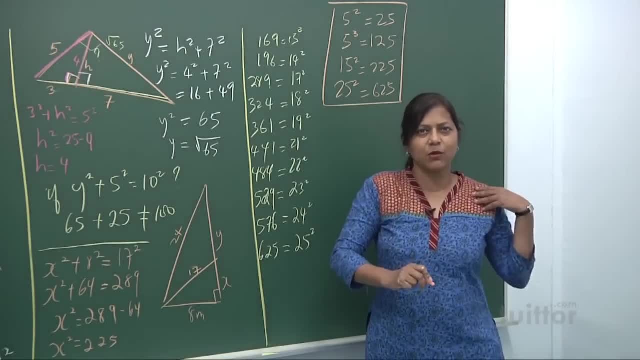 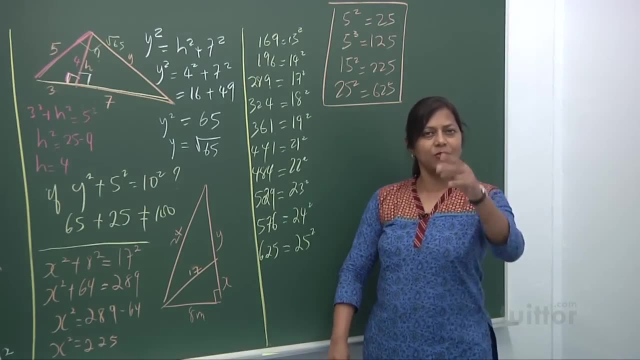 All right, And I know some rough youngsters. they feel so great To fight. All right, I hope you know one of them. To fight 15 squared 2 to fight. 25 squared 6 to fight Ah. 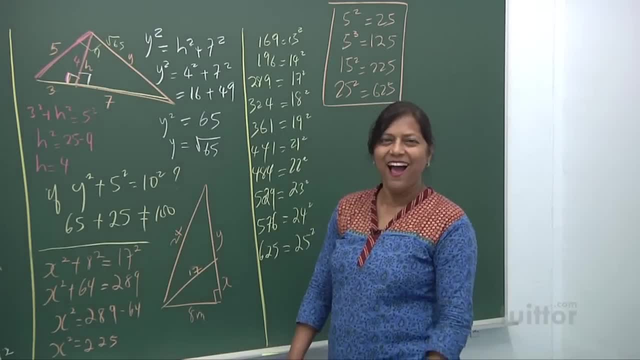 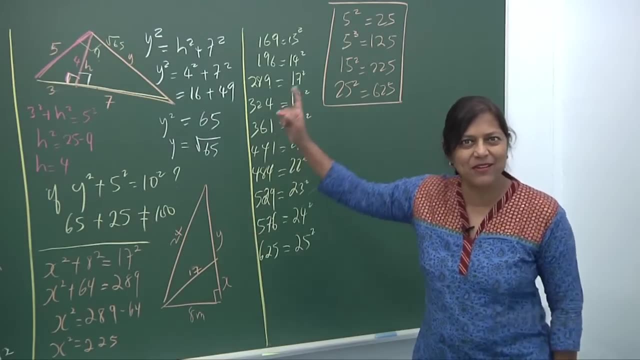 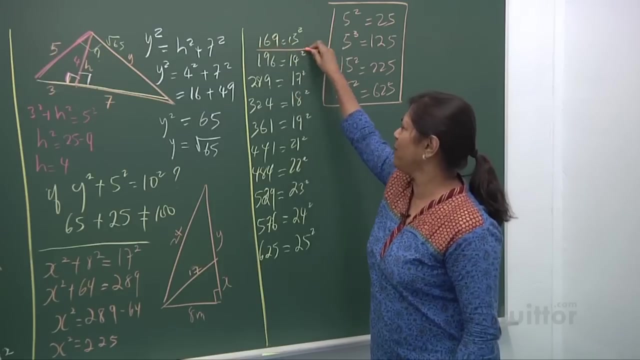 Gang fight. Run away. All right, Let's move on. This is just a package that you can remember and keep that secret. learning numbers, Just like here: I told you 69,, 169.. Here is 196.. In Singapore, what we do is we have a bus that goes down 169. that goes to you know. 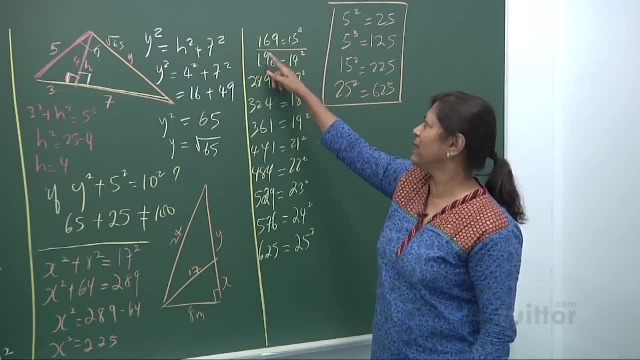 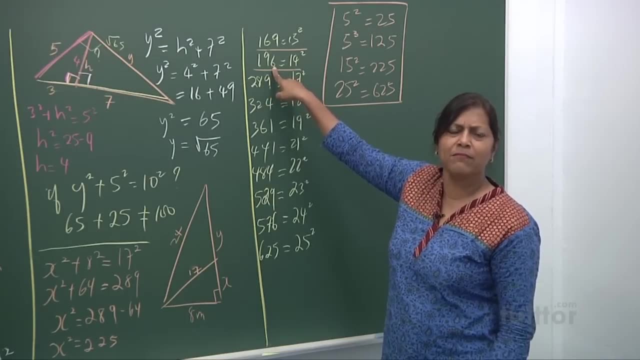 Yushun Sembawang area And I remembered I was supposed to go down to Jurong. you know, when I was a young girl And I took this bus 196.. I got confused because these two buses came at the same stop. 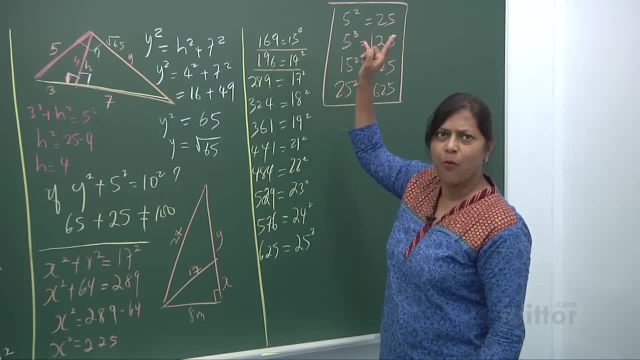 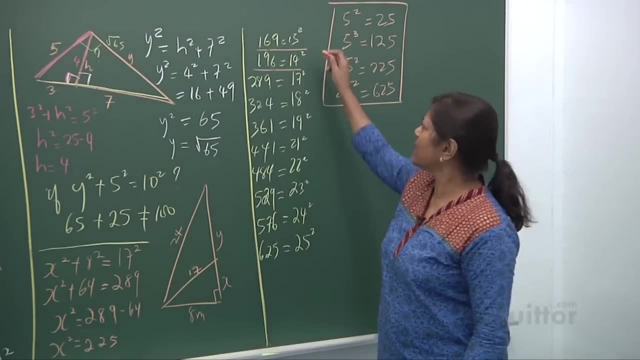 Oops, 196. And I ended up somewhere And then I realized, oh my God, it's supposed to be 169. Wrong bus, All right. So sometimes little stories, little anecdotes in your experiences can help you to make connections. 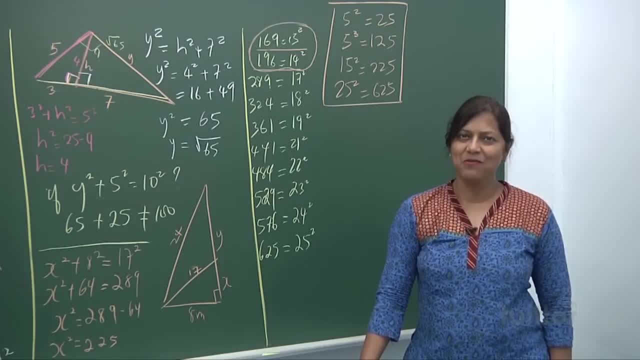 With numbers. All right, I'm sure you can connect with birth dates and whatever, All right, Okay. So let's look at this Now. you want to find out what is X. You've got X squared. This squared plus this equals a 17 squared. 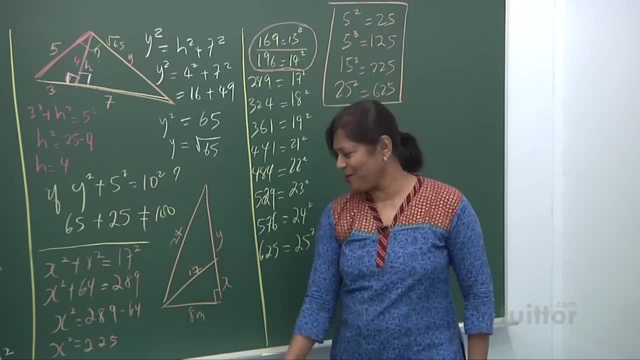 Your X is square root of two to five. What is that Fifteen Great? So your X is 15.. So you said: hey, you're 15.. And you're 15.. And you're 15.. You're 15.. 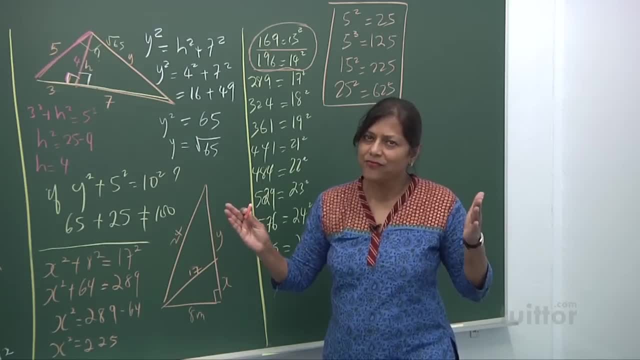 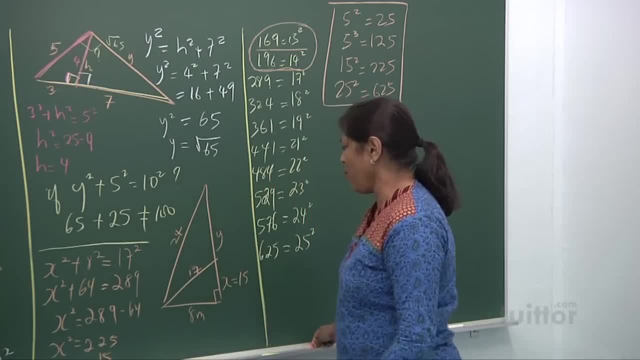 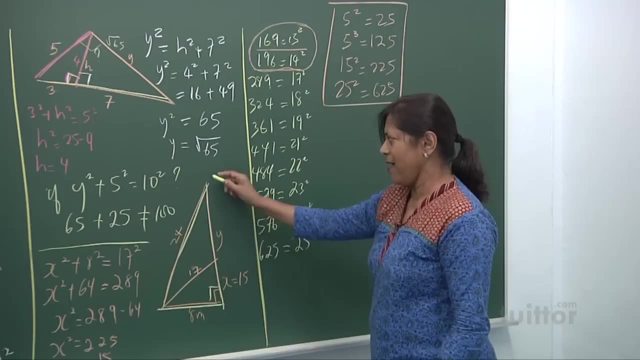 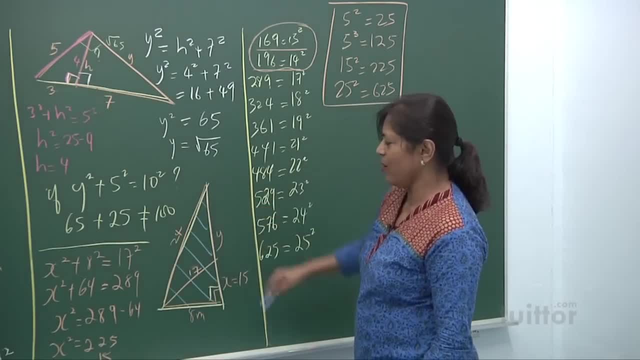 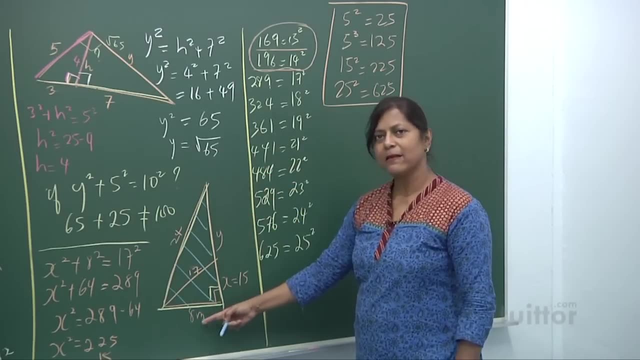 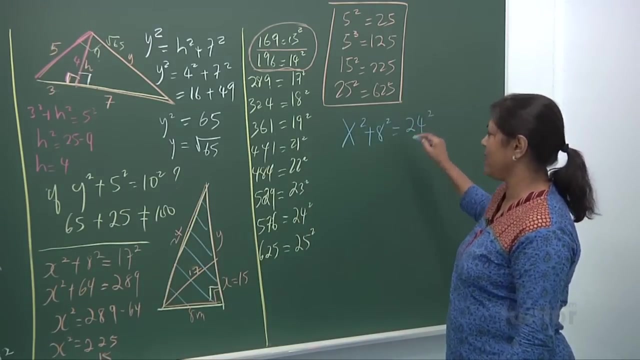 Now I'm looking at this big triangle. It's your hypotenuse, So this whole length I keep it as a big X. Big X plus X squared- All right, Is equal to 24 squared, And 24 squared you could get in your calculator for the moment. 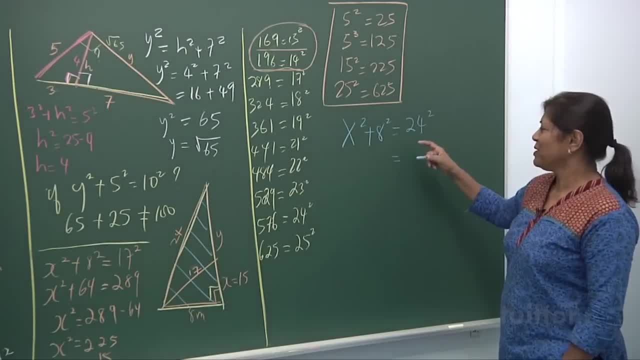 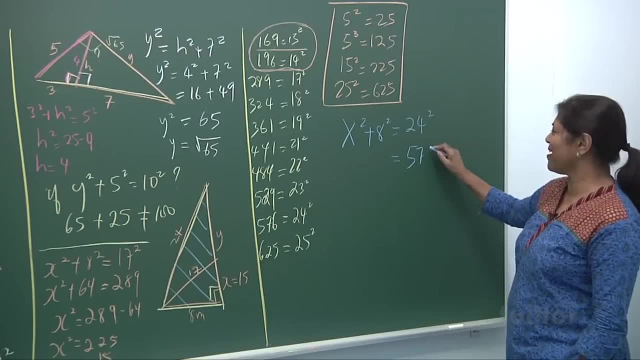 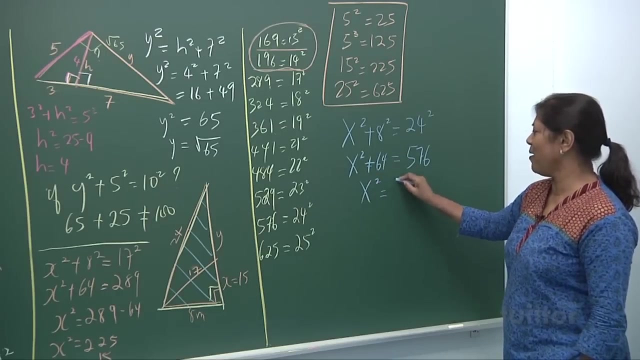 But I truly advise you to know your tables. 24 is near 25.. It is near the big gang fight. It's 576.. And this X squared plus 64. Bring the 64 over, You get a minus 64.. 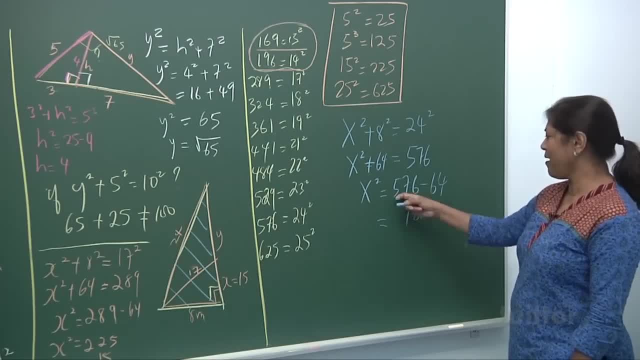 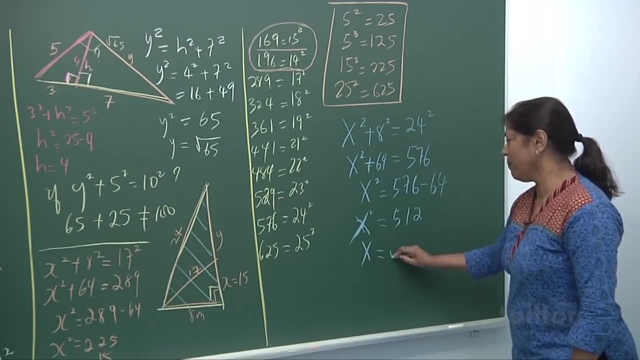 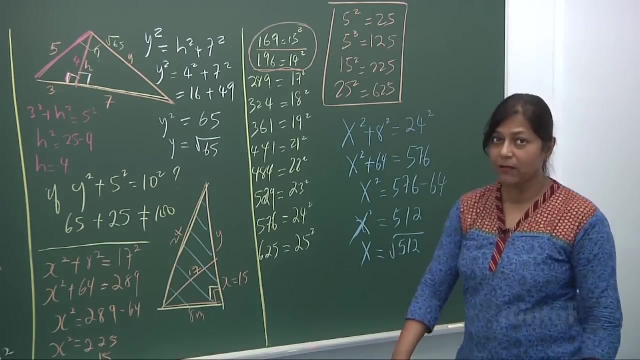 OK, 64.. 2., 1., 5. 2.. That's your X squared And, sorry, your X will be the square root of 5, 1, 2.. Now these are numbers that sometimes you need to help to get a calculator to help you find the square root of 5, 1, 2.. 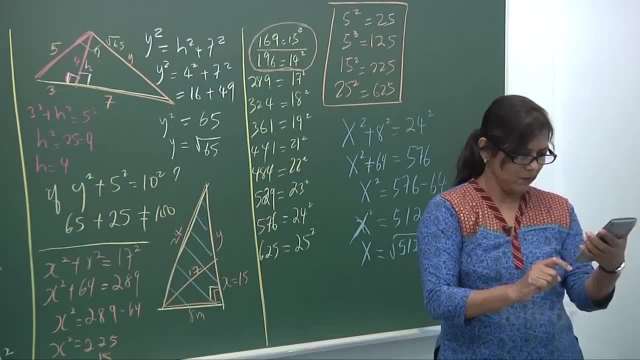 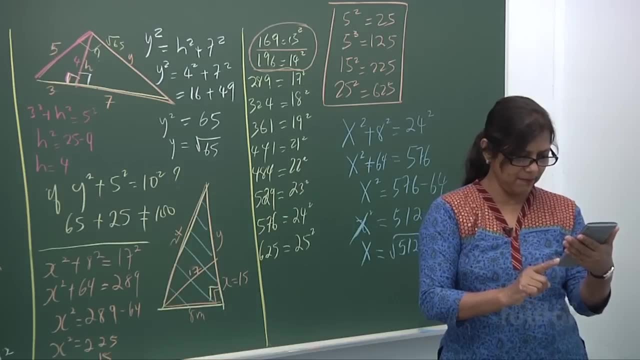 Look at the square root sign. Where are you square root? I've got to get that square root sign. Look at the shift button. Yup, I got it. Now get your square root Put down: 5,, 1,, 2.. 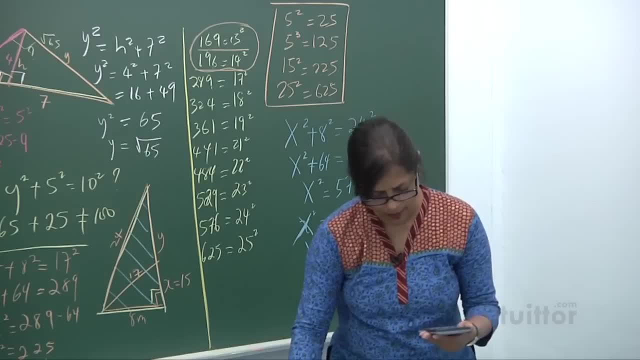 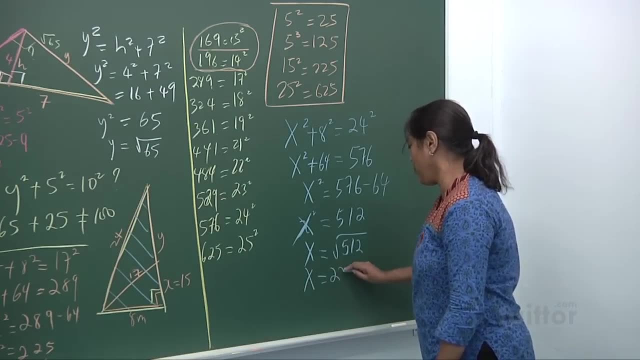 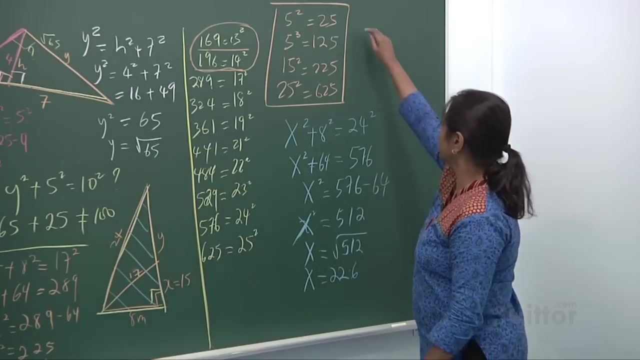 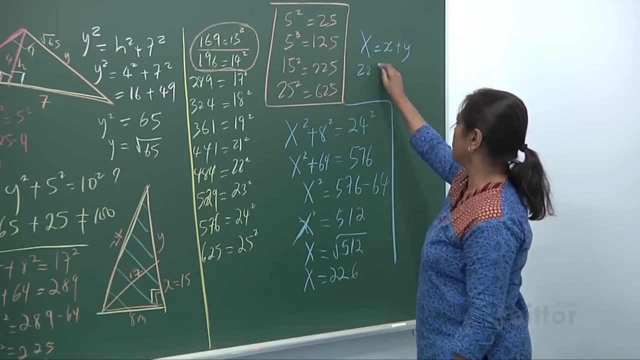 And press equal, You get 22.63.. So let's round out: X is 22.6.. And hence, as X is made of small x plus y, X is made up of small x plus y. Well, this is 22.6.. 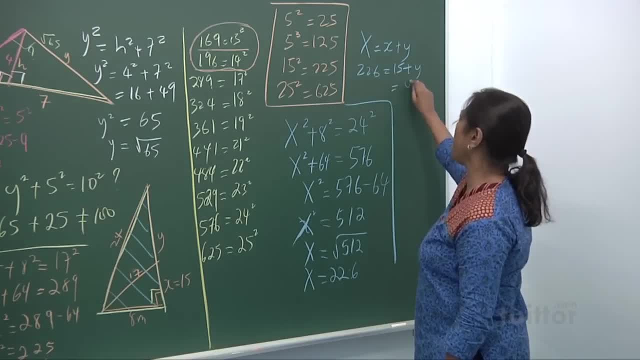 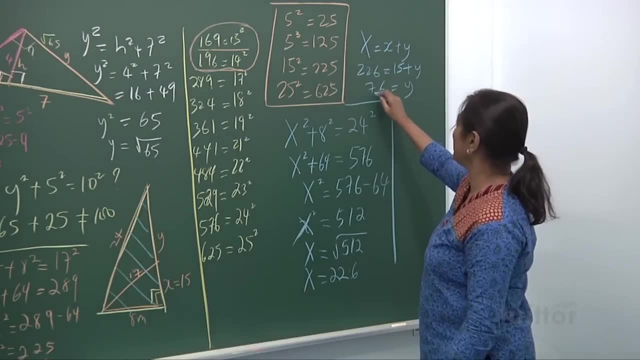 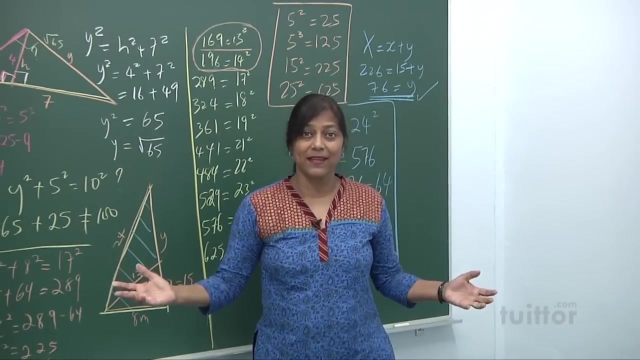 And that's 15.. So what is y made of 22.6 minus 15. You get a 7.6.. Ah, So you see, the use of Pythagoras is very easy, finding out length. 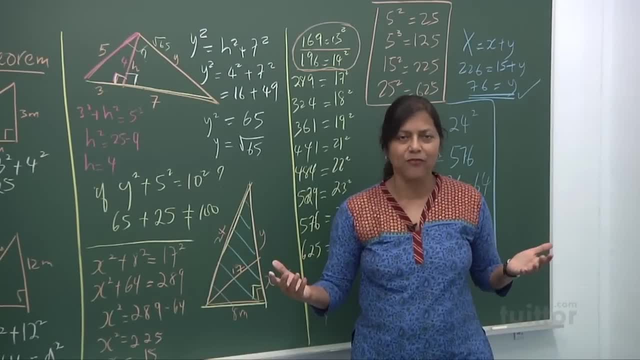 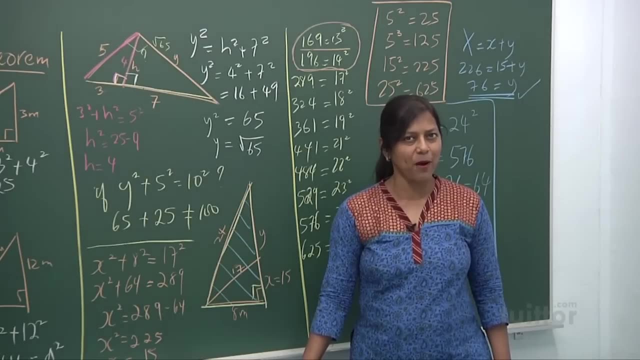 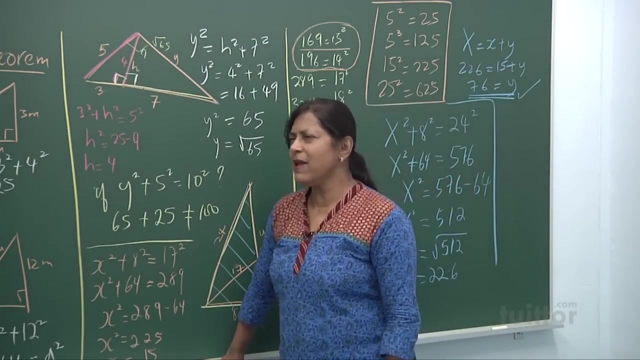 And its real measurement is the truth of numbers. All right, This amazing man, Pythagoras, I sometimes like to find out more about him. I like his name, Close to the name of Python. Pythagoras, His amazing strength. 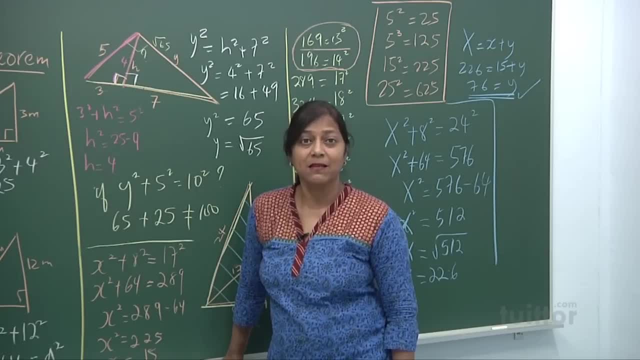 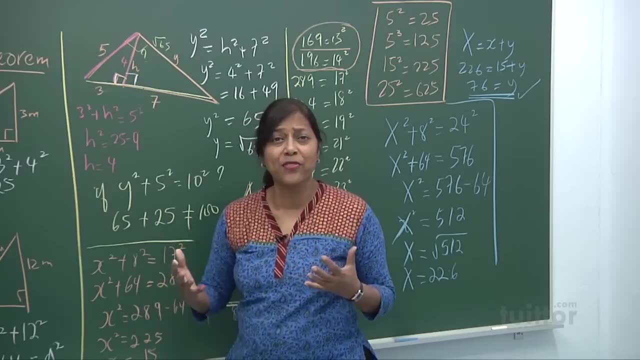 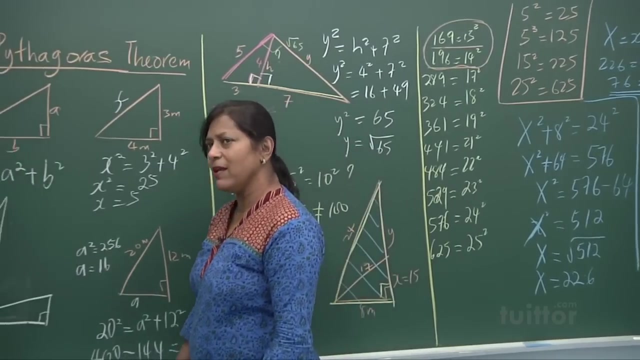 The amazing discovery that helped us discover more things in mathematics that we moved on. now, Because of these things, we can go into further measurements. All right, Now let's look at trigonometry Now trigonometry, In this case, at the level 1, we apply the first level. 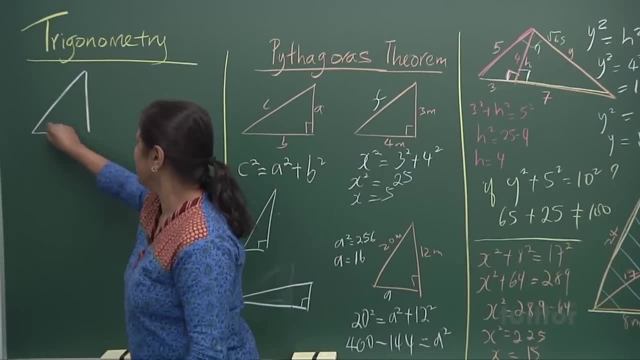 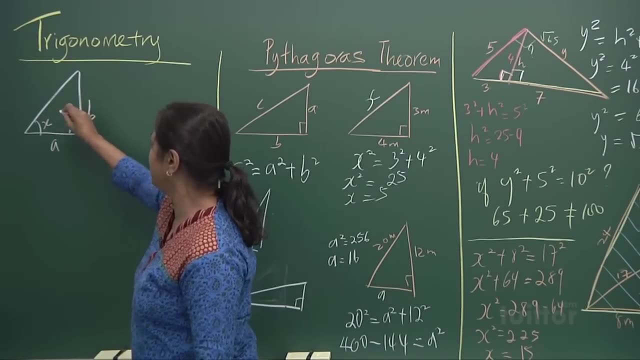 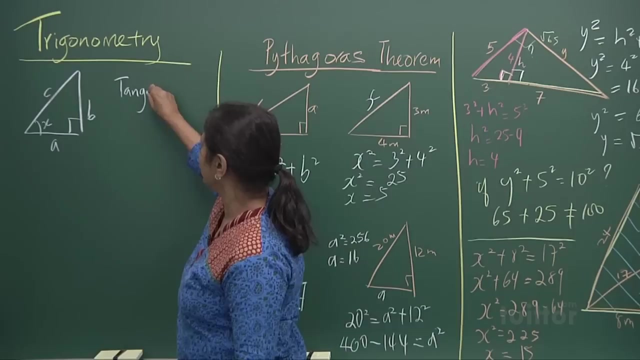 If it's a right angle triangle. Right, If you look at the right angle triangle. If you have an angle here, X And this is ABC. Now we look at tangent. All right, Tangent, the short form is 10.. 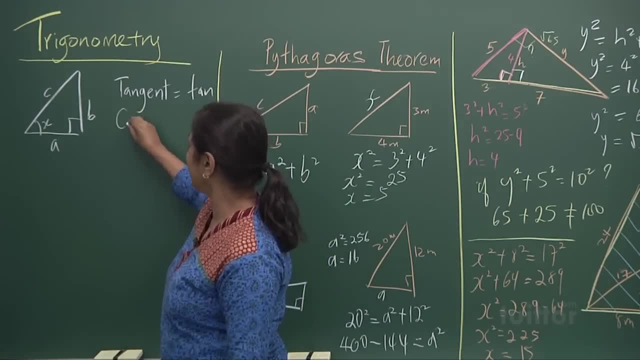 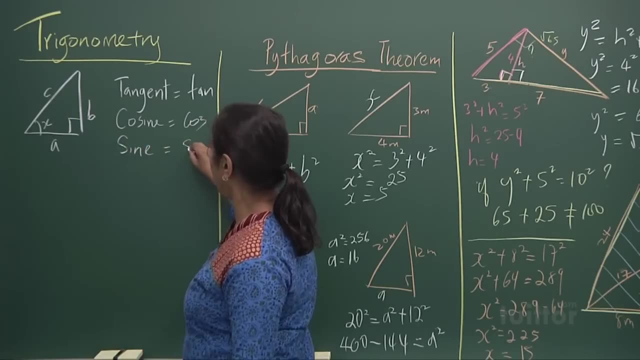 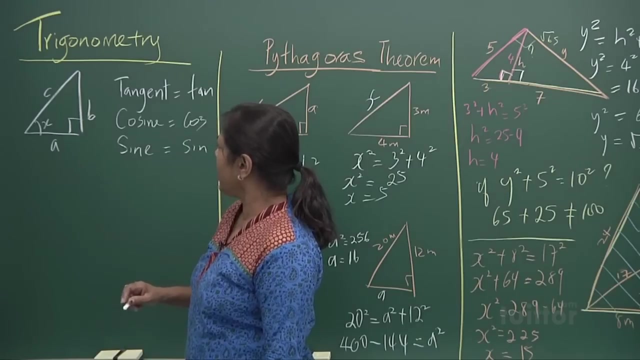 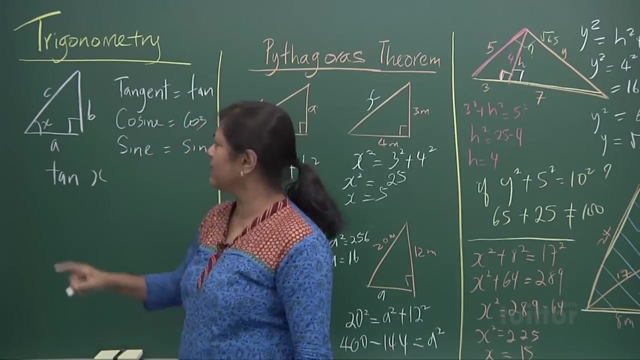 Short form Cosine. The short form is cos And sine, The short form is sine, Sin Like that Sin. All right. Now if we look at tangent, All right, Tangent X. Now I would like to say tangent is the opposite. over the adjacent. 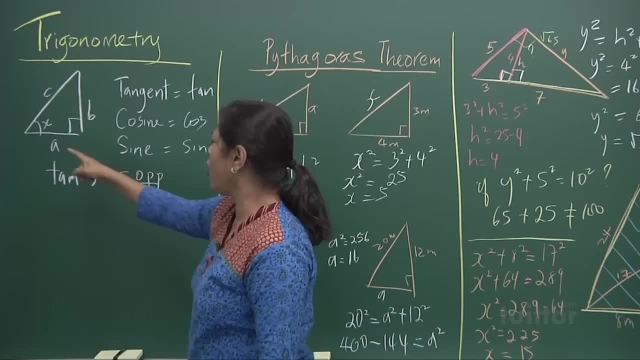 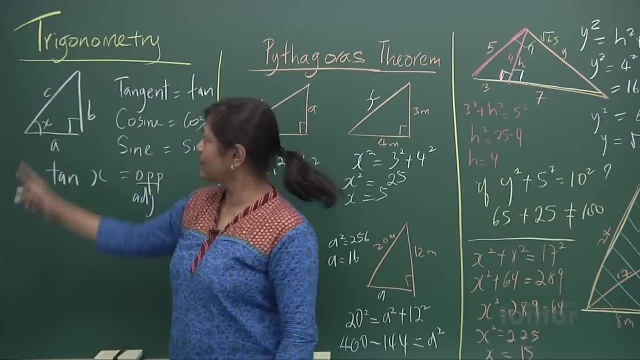 Opposite over the adjacent sine. Who is opposite? Well, this length is always going to be the hypotenuse. It's not going to change. That's going to be the hypotenuse. So tangent X is B over A. 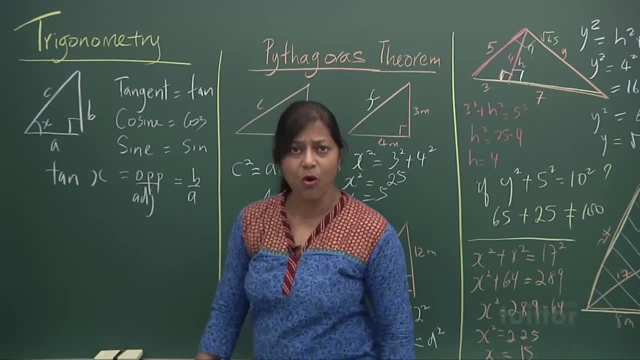 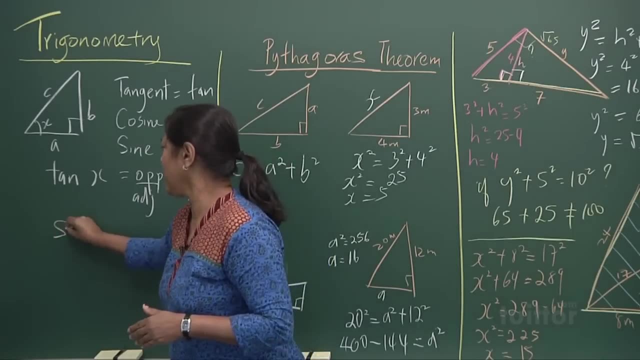 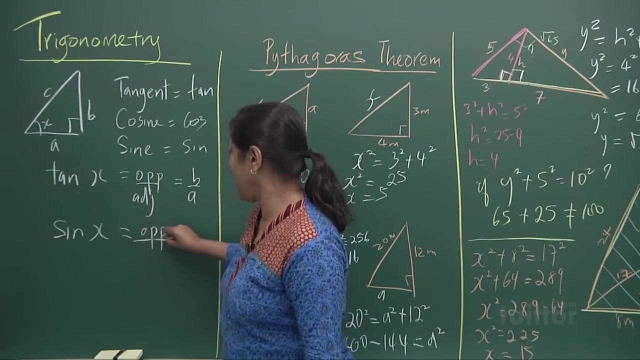 All right, The opposite side, Please don't get it wrong. Opposite X. Who are you? B over A? The next one? If you look at sine X, Sine is actually opposite, Actually opposite over the hypotenuse. 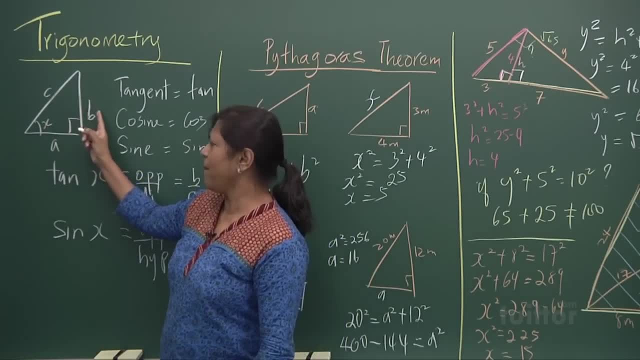 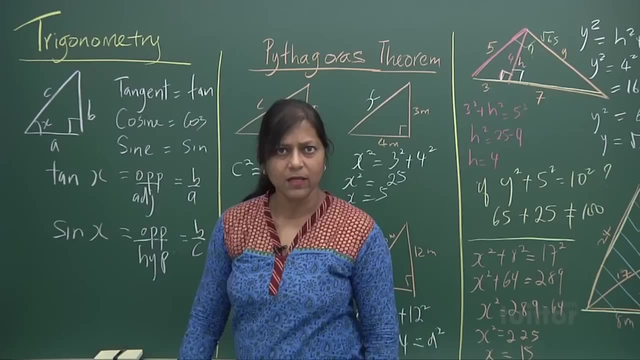 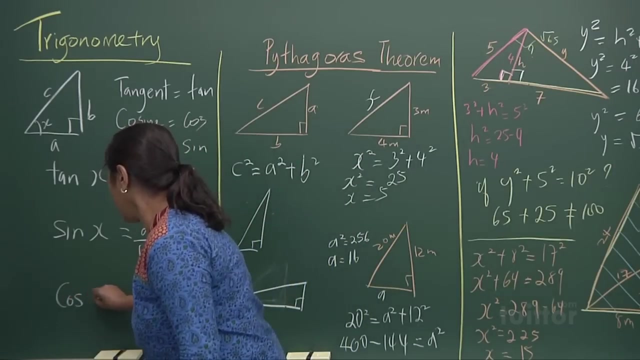 All right. And who is the opposite? The opposite side is B over C. That's your sine. The rule. Sine is opposite over the hypotenuse. And for cosine, cosine X is adjacent Adjacent. What does it mean? 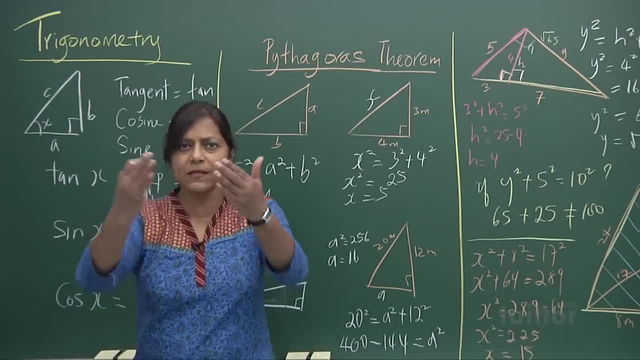 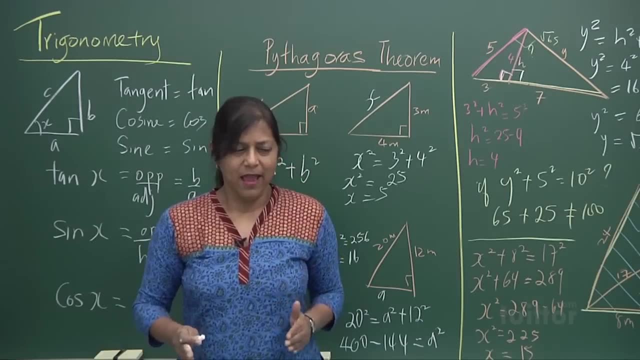 Beside you, Adjacent to you. When you say opposite, it's across you. I'm opposite of you, Right across, I'm sitting across, Adjacent to you, Maybe your mom, Maybe your dad, Or maybe your friend. 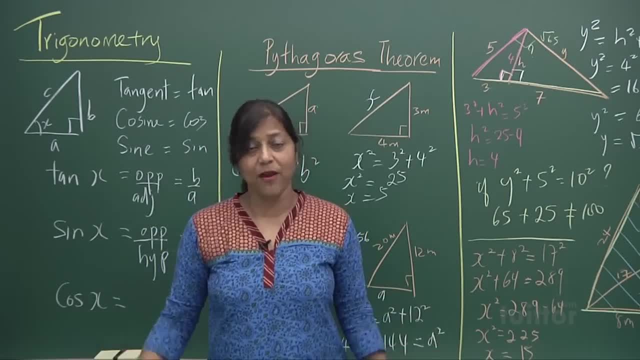 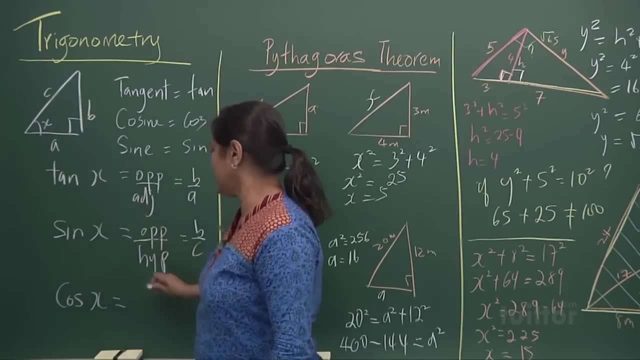 Your best friend, Or your girlfriend Or your boyfriend. Whatever friend Adjacent Next to It can be the right, It can be on the left, So adjacent to cos, The adjacent will be an A. Let me write here first. 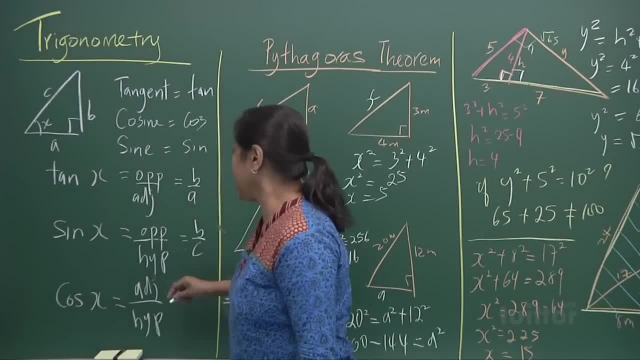 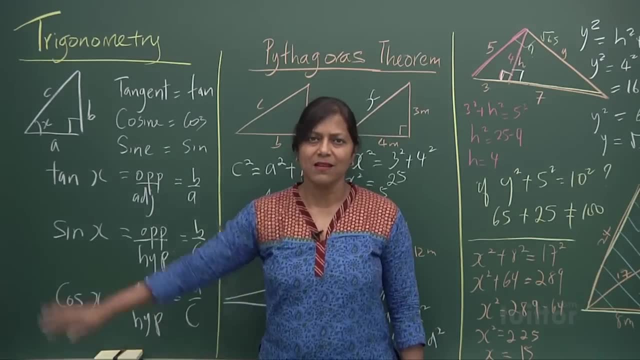 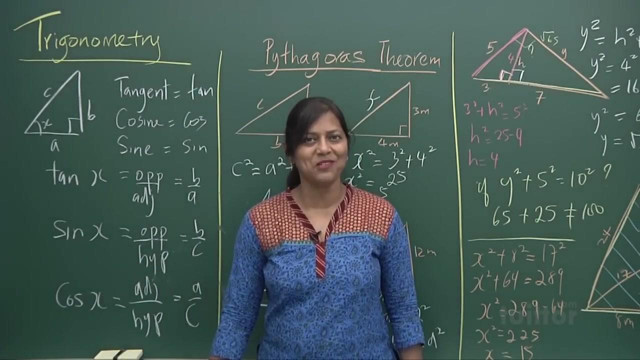 Adjacent over the hypotenuse And the adjacent is A over C And I'd like you to be familiar with these names, The formulas, Alright, And we will then go into more sums to understand trigonometry. I hope you've got your Pythagoras in you. 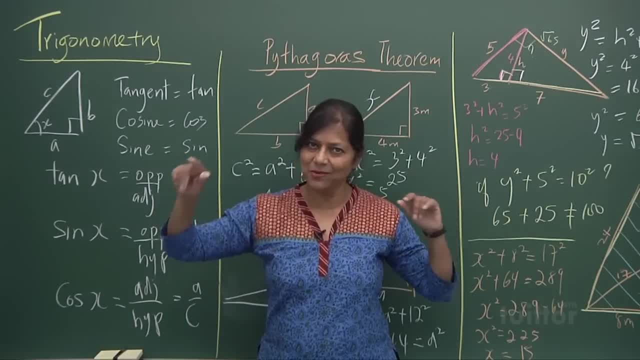 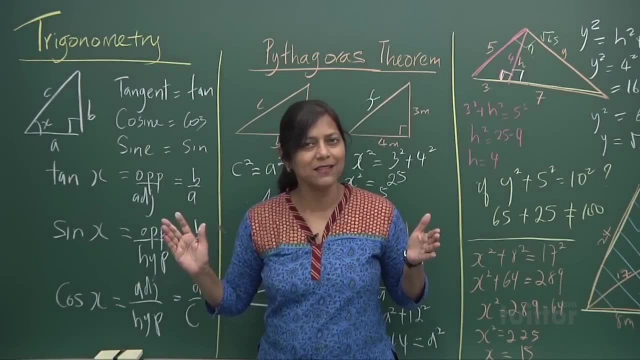 A squared plus B squared is equal to C squared, And the bigger side of the triangle is called the Hypotenuse. Is it Hypotenuse? Yes, Not what it is supposed to be. Have fun And we'll have more sums.